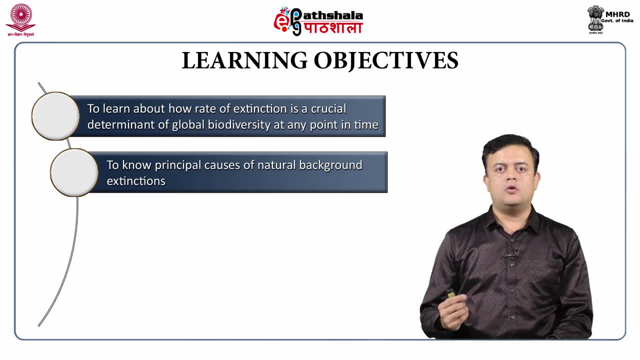 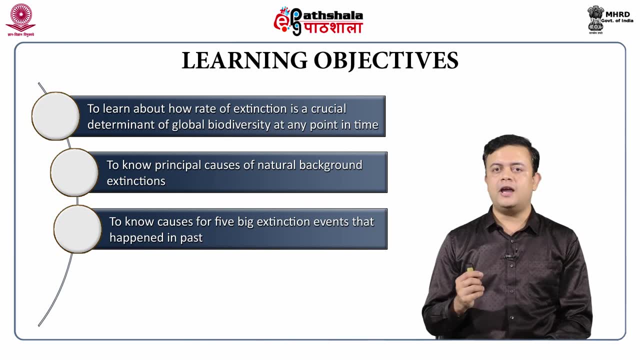 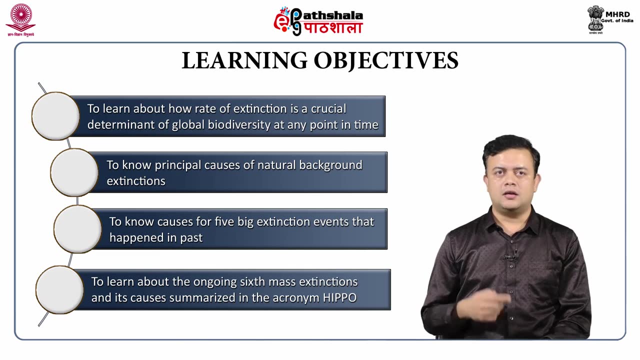 To know about the principal causes of the natural background extinction. So what causes this background extinction that we will come across this module To know the causes of the major five extinction events. So let's start with the learning outcomes. So we will coincide with the five extinction events that happen in the past and then we will learn about the ongoing six mass extinctions that summarized in the acronym HIPPO. 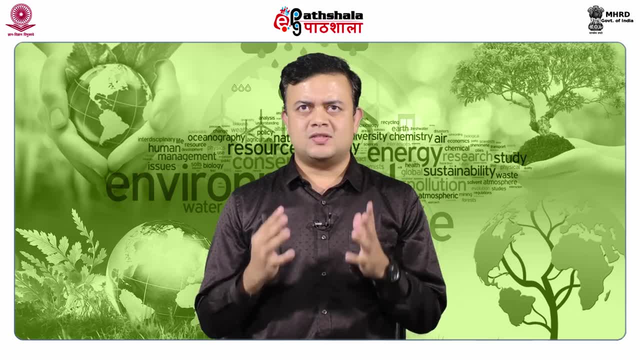 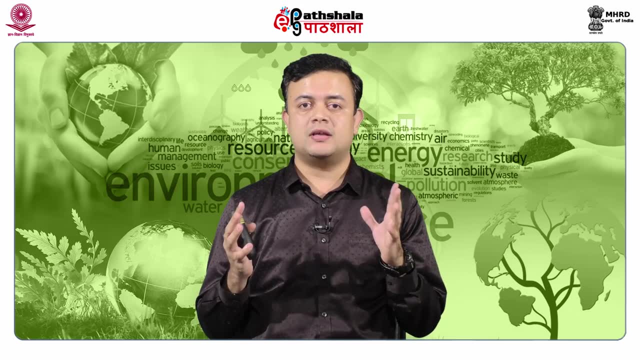 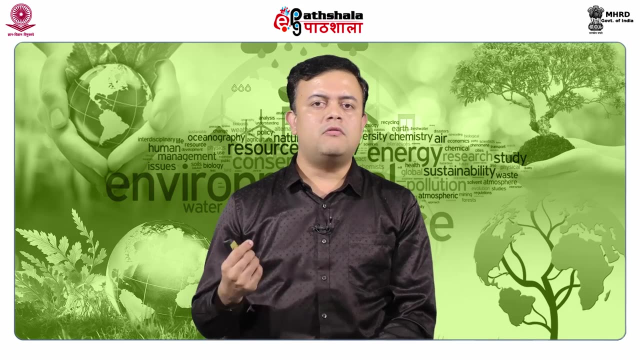 So the introduction is that at present there are like 10 million to 1 trillion all species that are currently extinct, that is, currently living on the planet Earth. However, we know only have very little bit of this. only there are 2 million named species. 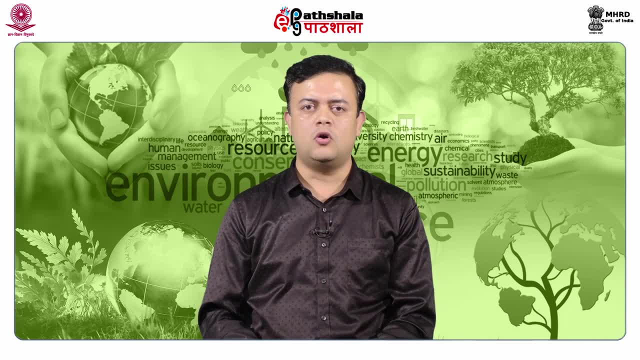 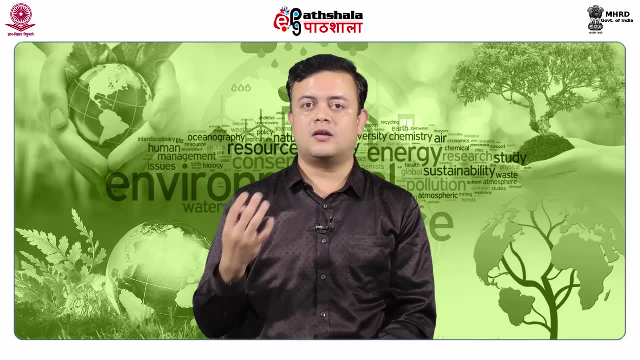 So vast majority, almost like 0.001% only we know. So the rest, 99.99%, remain to be documented And there is a huge crisis in this world that many of the species will go extinct even before the humanity could ever document. 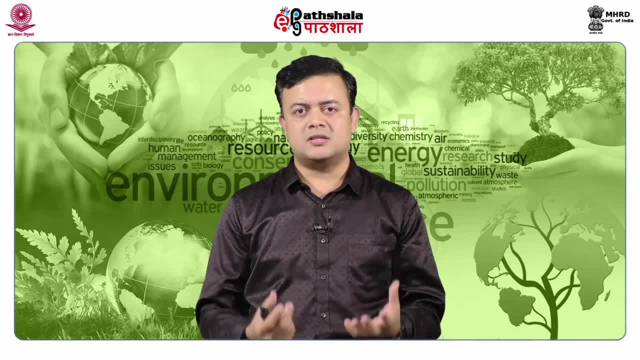 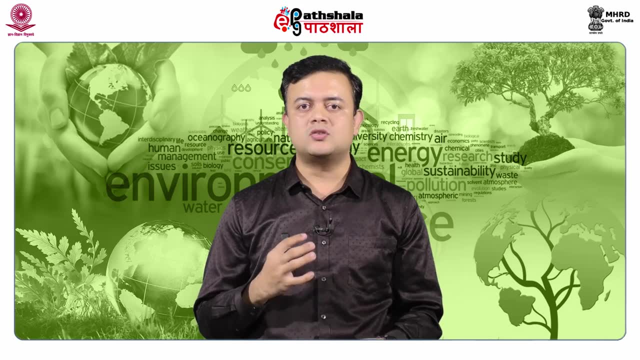 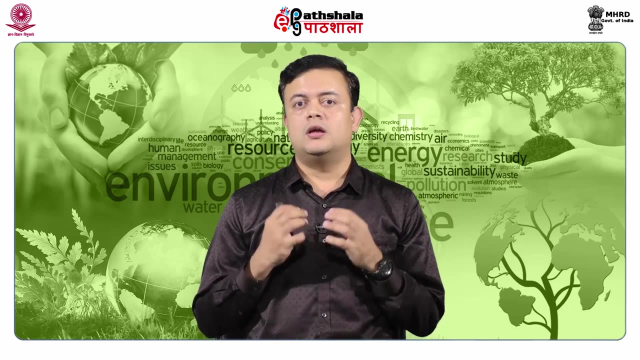 characterize these species. One of the common misconceptions in my students, as well as for the general public, is that majority of species extinction is caused by human activity, the anthropogenic activity, which is incorrect. Why it is incorrect? Because geologic time or evolutionary time scale. 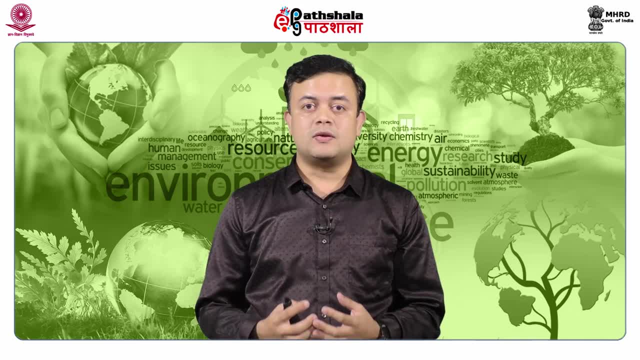 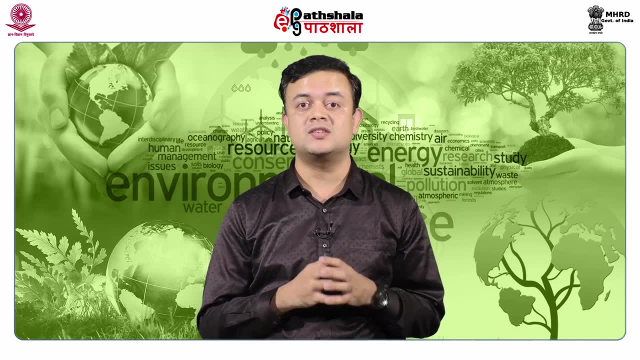 is immensely deep. The earth is 4 billion years old, 4.5 billion years old, where the life on earth is only 4 billion years. So 4 billion is such an immense time where our own species, the Homo sapiens, 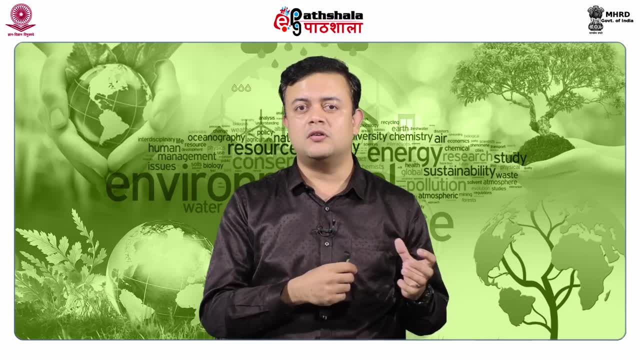 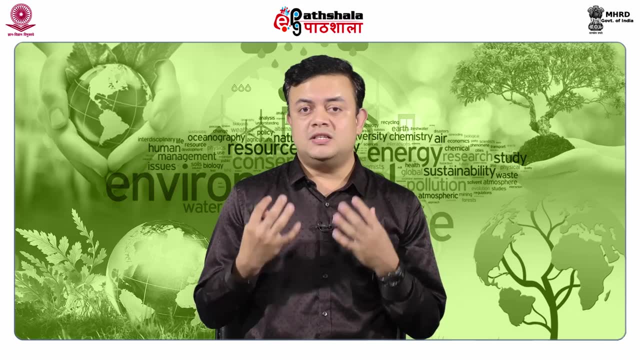 you know originated in the planet earth only around 300,000 years back, which is comparatively a recent phenomenon. So you know, almost 99% of the whole extinction event happened in the planet earth, happened even well before the human beings. 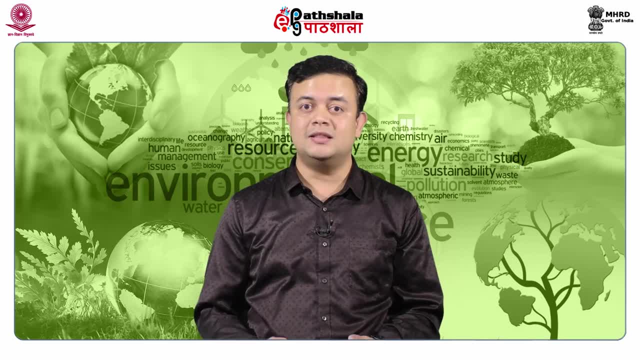 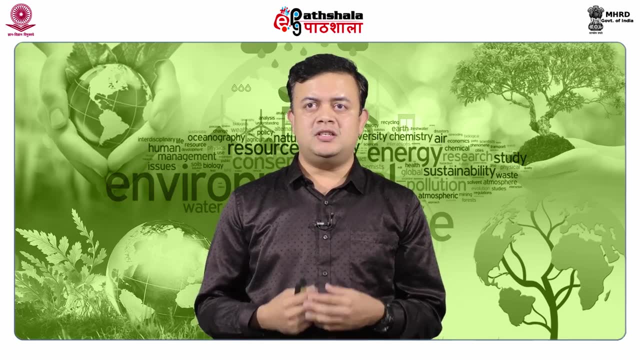 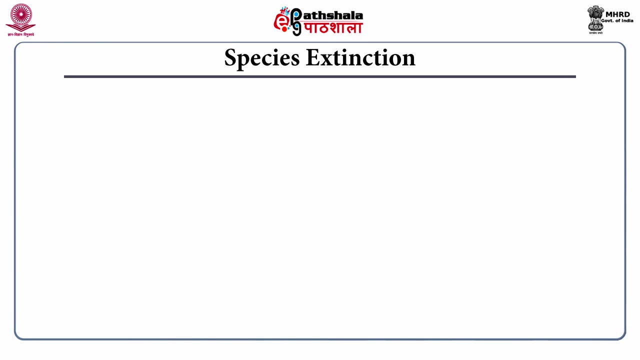 came to existence in this planet earth. So it's not the case that it's all anthropogenic. So it's estimated that more than 99% of all species that ever lived on this planet have gone extinct. So what is species extinction? So extinction, or also called species extinction. 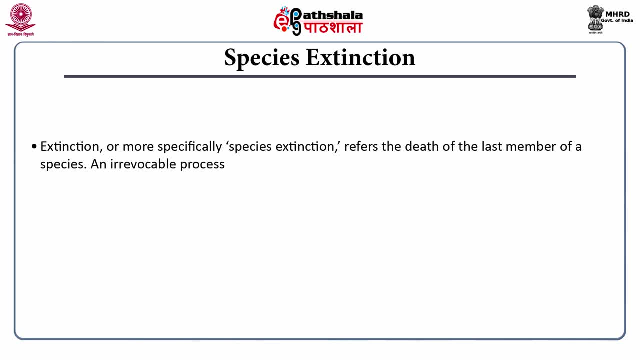 refers to the death of the last member of a species And, as you know, this one is a worldwide phenomenon. So the last member, the death, should be the end of the whole species. So it is something like a death, as you can see, an individual's death. 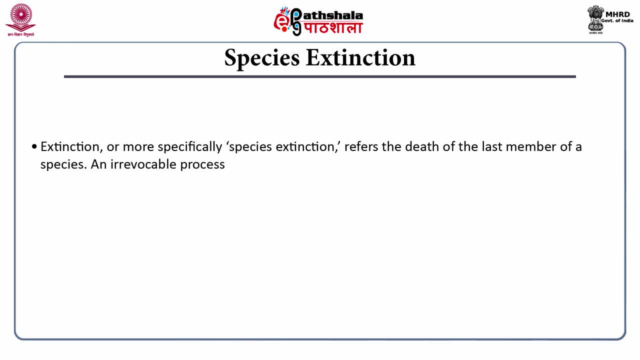 It is irrevocable. You can never go back to the life again. Similarly, once a species goes extinct, it's impossible to you know resuscitate it. So it's impossible to you know resuscitate it. 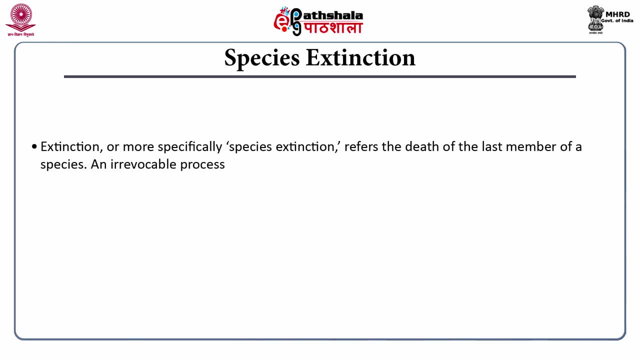 So it's impossible to you know resuscitate it. So it's impossible to you know resuscitate it, That particular species back to the life again. So it's an irrevocable process. So, as the definition is centered about the species, 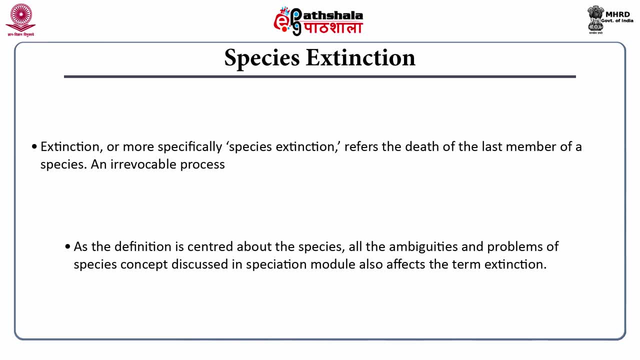 and of course the species definition, as we will see that in the Modulon Speciation is very tricky and very subjective. the interpretation, what constitutes a species? So all the logical as well as philosophical problems associated with the concept of species is applicable for the species extinction as well. 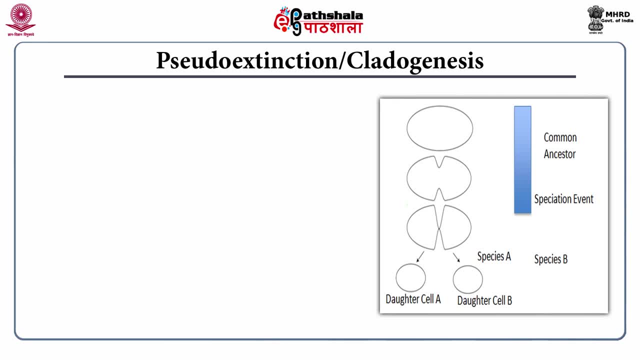 So the species extinction can be contrasted with yet another phenomenon called pseudo-extinction. So what is a pseudo-extinction? It is analogous to the binary fission. See in the case of binary fission. so it is like one bacterial cell. 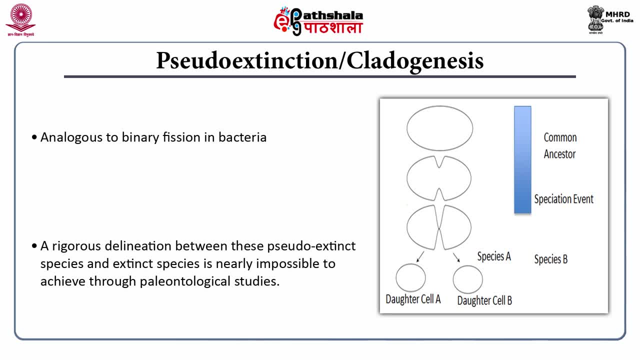 that is dividing into two bacterial cells. So that is called. the one parent cell divides into two daughter cells. So similarly, one contiguous population of one species somehow gets separated by you know a geological phenomenon, For example a mountain range. So mountain range separates the same parent population. 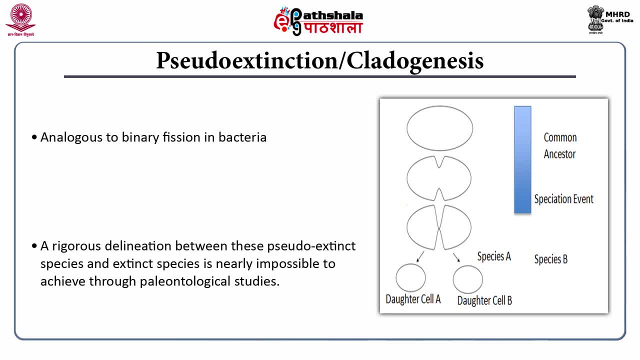 into two, to form two daughter populations, And each of these daughter populations diverge into two different species, Then what will happen to the parent population that is not existent? So you can never say that the parent population when extinct to produce a daughter population. 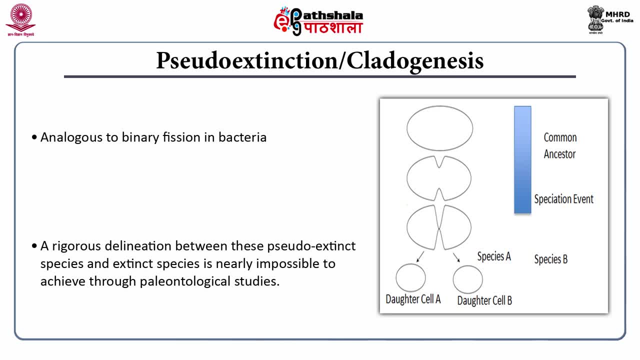 That is incorrect to say that way. So that is not really a species extinction. That is simpler a cladogenesis, the formation of a new species from, you know, pre-existing species. So that is called pseudo-extinction. So lifespan of a species. 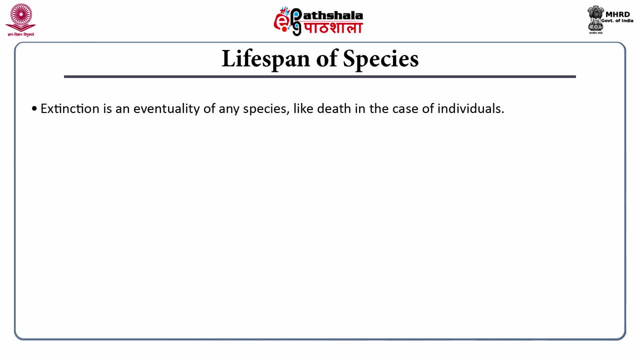 So how long will the species live? Again, it depends upon various species and various lineages of the tree of life. So, for example, the average lifespan of a species is determined to be 3 million to 10 million years. So that is the average lifespan. 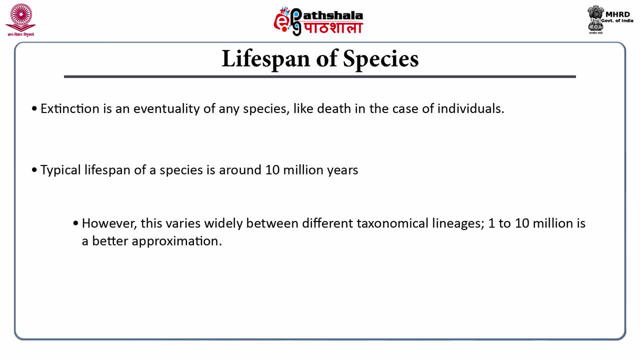 Again, it's an average estimate. You know it's a range And several species are very short lived, only a few thousand years, While a few species are extremely long lived. those extremely long lived species are somehow- sometimes we refer it as living fossils. 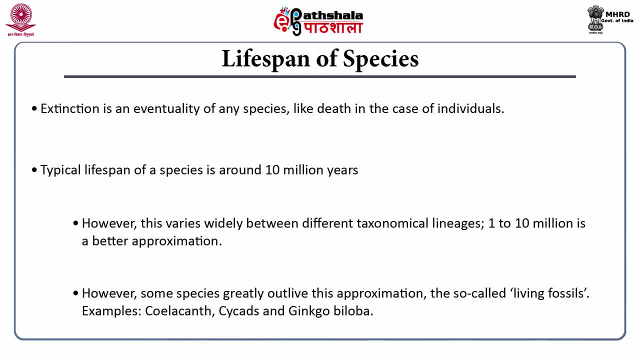 One example is Ginkgo biloba, the plant which has been in existence since Carboniferous, almost 200 million years old, Or silicon, the fish, the lungfish silicon or cycad, the plant. cycad is an example of a living fossil. 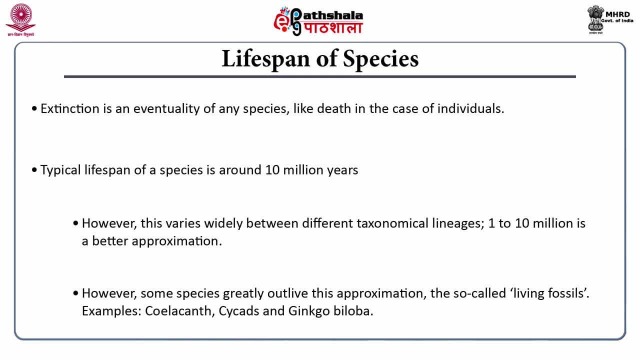 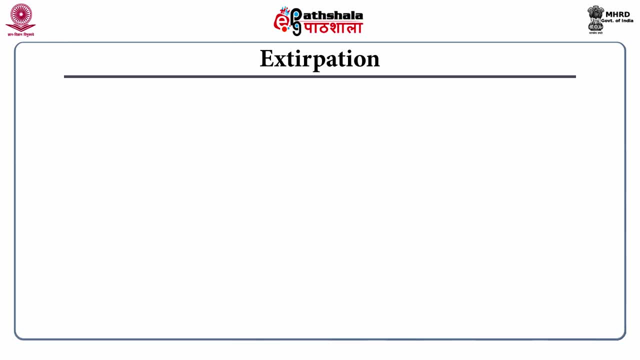 which greatly outlived the approximation of, you know, around 10 million years. The species extinction can also be contrasted with yet another phenomenon that is called extirpation. So extirpation is a local extinction, So extinction of a particular species. 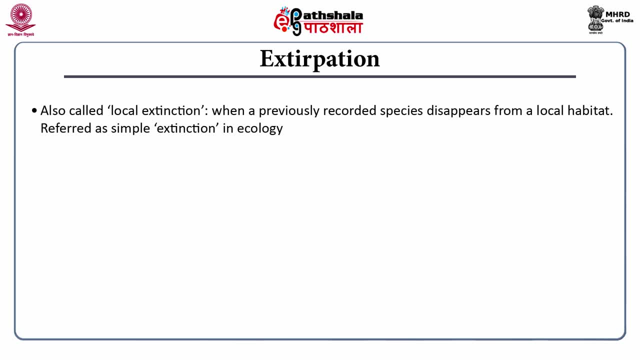 from a local community or a habitat, For example in an island, the last surviving species of a bird goes extinct. That is called local extinction or extirpation, But in the ecology the term extinction is used to refer the local extinction. 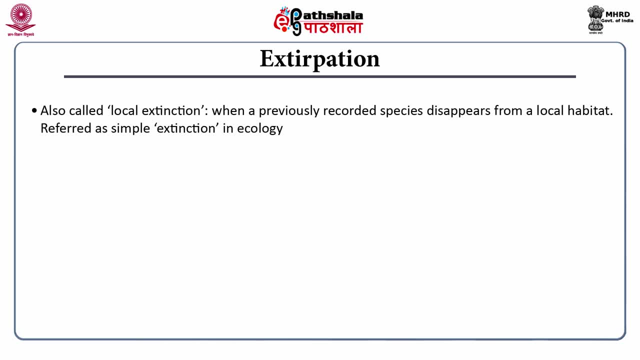 So there is a subtle difference of the term extinction used in ecology as well as that used in the other sciences. So extinction of one species, especially keystone species, have huge repercussions on the rest of the ecological niche in which the extinct species was part of. 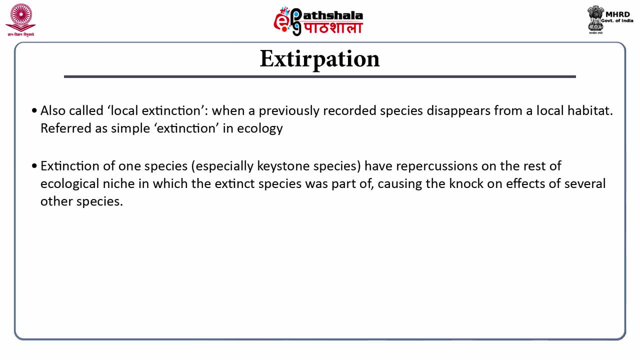 causing the knock-on effects on several other species of the community. One example is that consider elephant in a savanna ecosystem, for example, that in Africa. So as the African elephant is a keystone species, it actually eats the bushy plants as well as the trees. 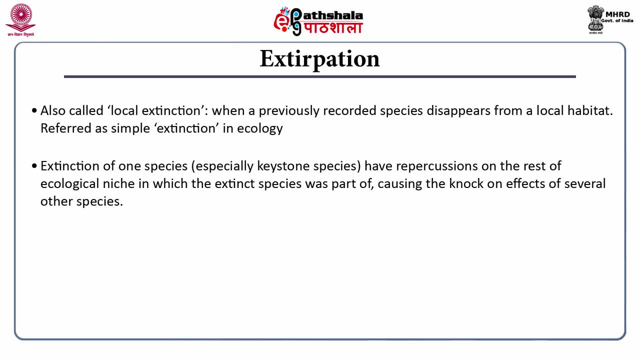 It's very essential that the elephant needs to be in the savanna. So if the elephant goes extinct, the savanna is no more a grassy savanna. It will be a bushy land. It will be converted into a forest, where most of the community structure of the savanna 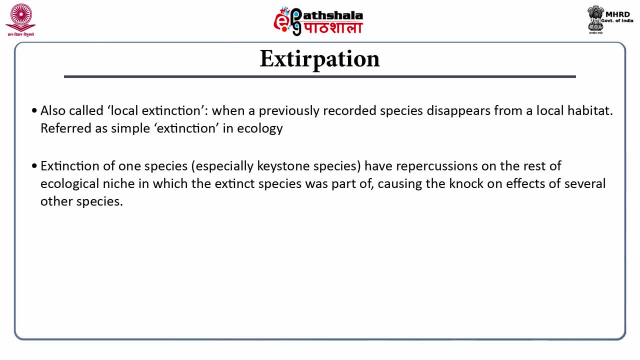 will be totally eclipsed And most of these species will go extinction, the local extinction. So it will knock on a chain reaction of various local extinctions. So there is a phenomenon in the extirpation. So if the species is endemic, 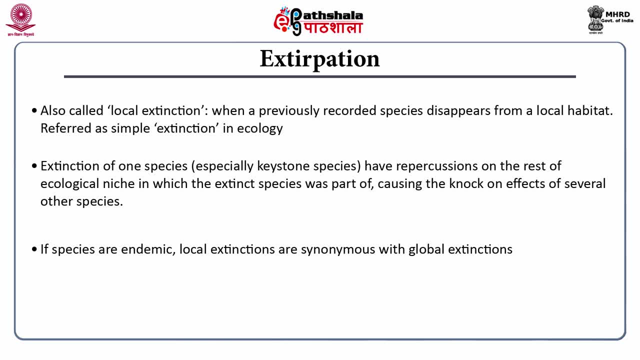 so that means it is not found nowhere else in the world, only in that particular location. For example, you can consider an island and that particular species is found only in that particular island. So local extinctions of that island, so local extirpation of that species in that island. 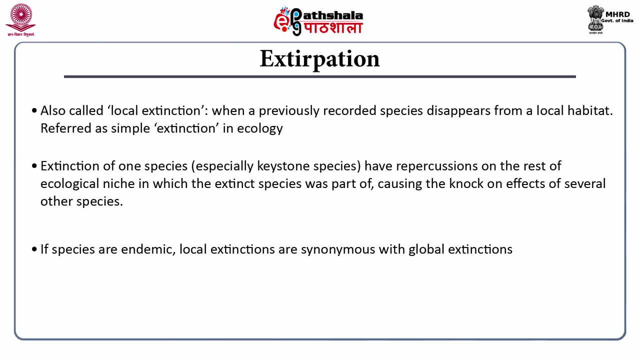 means death of that species in that island. It's synonymous with the global extinction because that species occurred nowhere else in the world. So in terms of endemic species, extinction from a simple locality- for example a fish going extinct in a lake- if that's an endemic species that's found only in that particular lake. 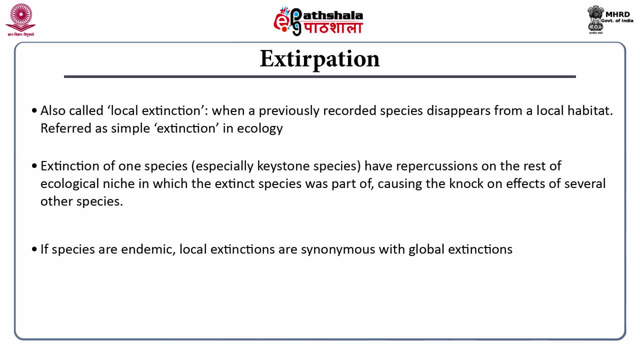 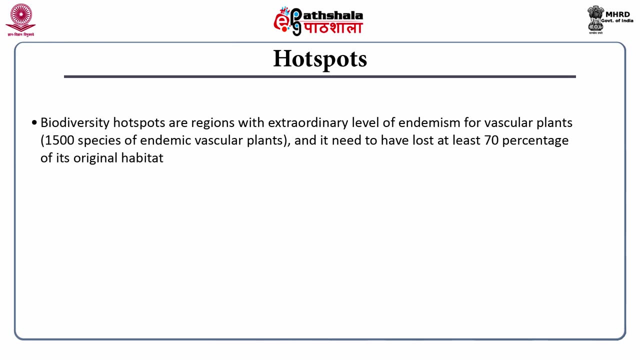 it's synonymous with the global extinction. So that is the reason the conservation programs are often biased towards hotspots, the areas with high endemic organisms, for these reasons. So what are the hotspots? These are biodiversity hotspots or regions with extraordinary level of endemism. 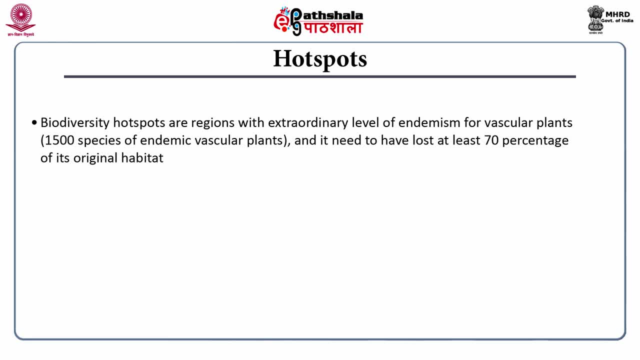 for the vascular plants. So by definition the biodiversity hotspot is skewed towards vascular plant diversity, So it should have at least 1,500 species of the endemic vascular plants for the biodiversity hotspots And it needs to have lost at least 70%. 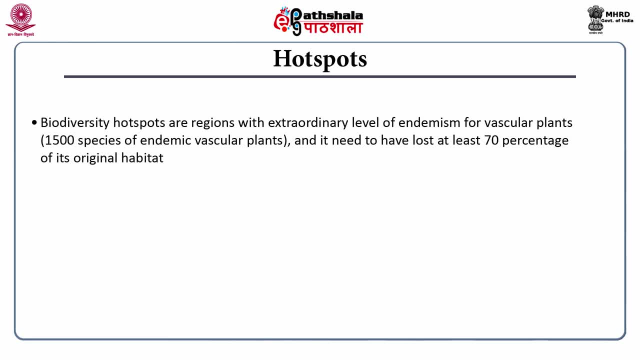 of its original habitat. So these locations, the hotspots, needs to be under tremendous anthropogenic pressure to call it as a hotspot. So that is why these hotspots are the main concentration, main objectives for most of the worldwide conservation program, because these hotspots are tremendously under pressure. 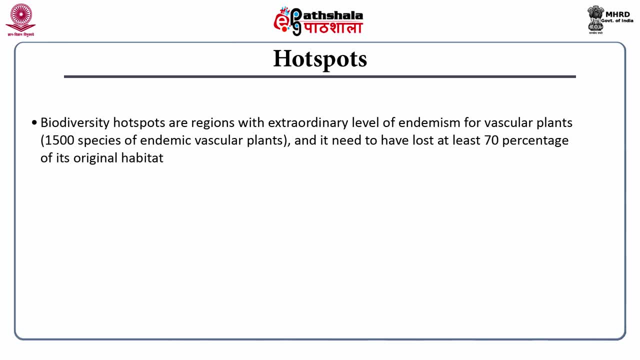 from the expanding human population. While the hotspot criterion is based on endemism and loss of habitat, it's skewed towards the vascular plant. As I told you, it needs to be having 1,500 species of the endemic vascular plants. So vascular plants are the plants with xylem and phloem. 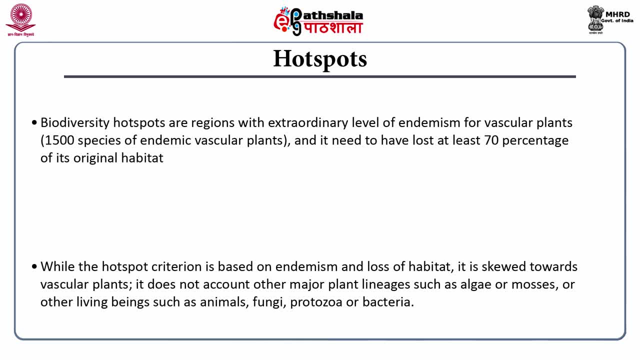 as you see, the higher plants, But it does not take into consideration of lower plants, For example, cryptogams, algae, mosses, ferns, other living beings, animals, Even though a particular location have a huge number of animals. 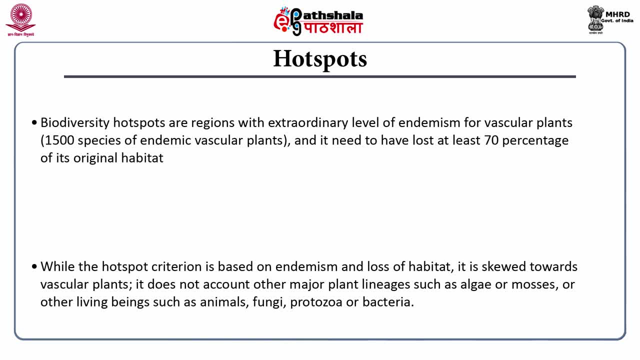 you can never call it as a hotspot. So that is an inherent problem. Fungi, protozoa, bacteria, fungi, the virus: nothing is taken into consideration while defining the term hotspot. So there are a number of hotspots in the world. 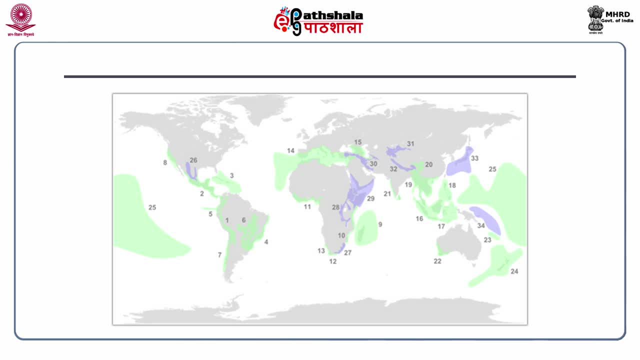 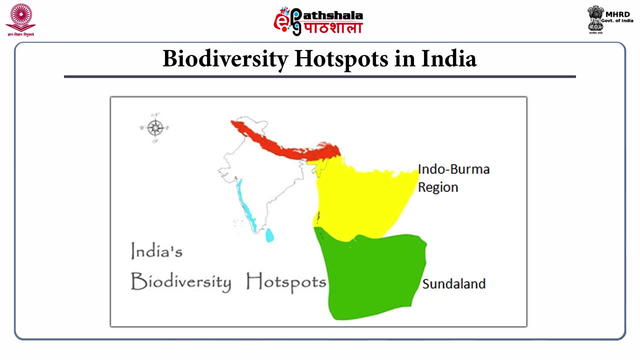 out of which four are in India. Four hotspots in the Indian subcontinent are the Himalayas, which is later added. The original three hotspots were Western Ghats in South India and Indo-Burma region, that is, on the northeast of India. 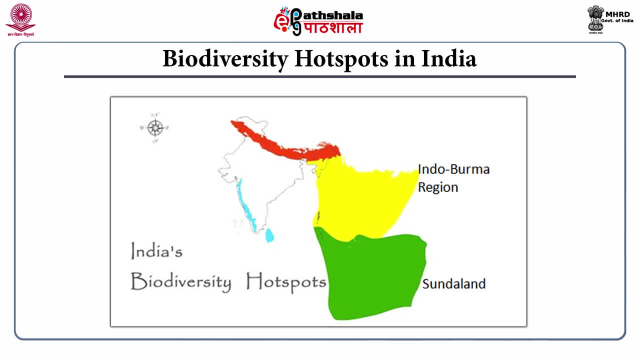 as well as including the island of Andaman and a little bit of the islands. you know the Nicobar island is part of the Sundaland. That is yet another biodiversity hotspot. So we have got now four hotspots in India. The fourth one, 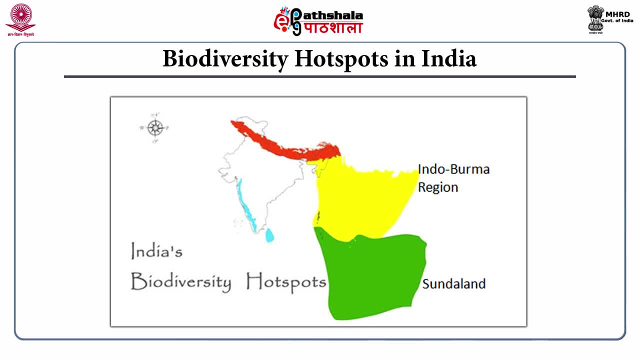 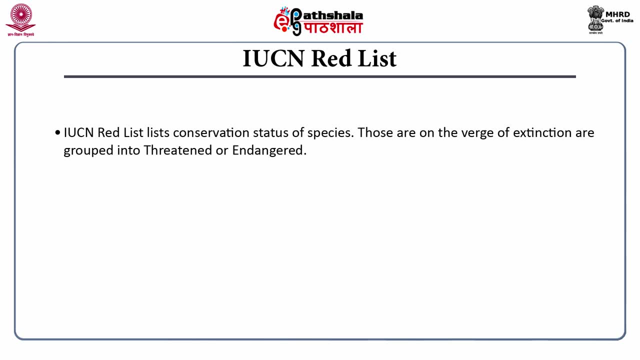 lately added is the Himalayas, including the east too, as the whole Himalayan region is the fourth biodiversity hotspot. So IUCN have come up with a red list that is endless. the conservation status of species. So is the species vulnerable, threatened? 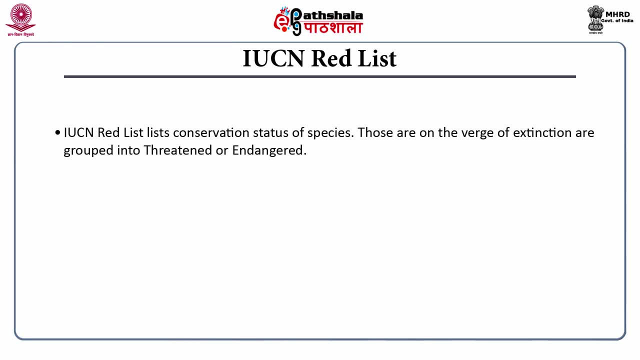 or extinct. You know all these different labels are being given to different species that is on the verge of extinction in the IUCN red list. So those that are on the verge of extinction are grouped into threatened or endangered. So these species are in imminent threat of extinction. 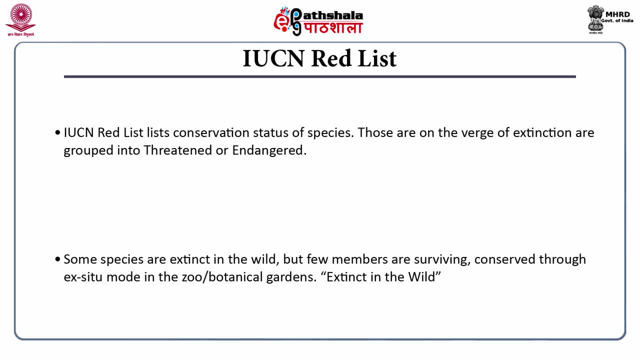 So some species have gone extinct in the wild, So only surviving members of those species. you can see it in, you know, the zoo or botanical garden, the so-called, you know, ex-situ conservation. So those species are called extinct in the wild. 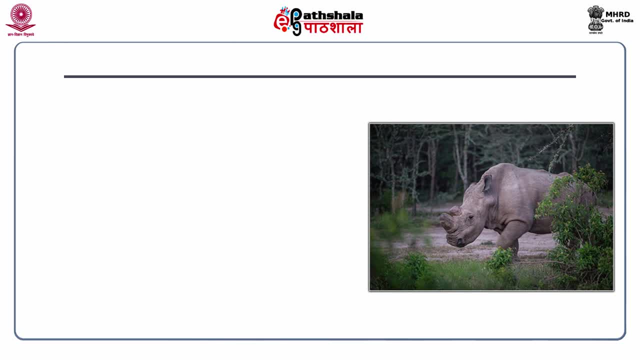 One example is a white rhino. The last month, so 19th March of 2018, a few weeks from today, so the world's last surviving male, you know, the white rhino has gone. I mean, the rhino has died in a conservatory in Kenya. 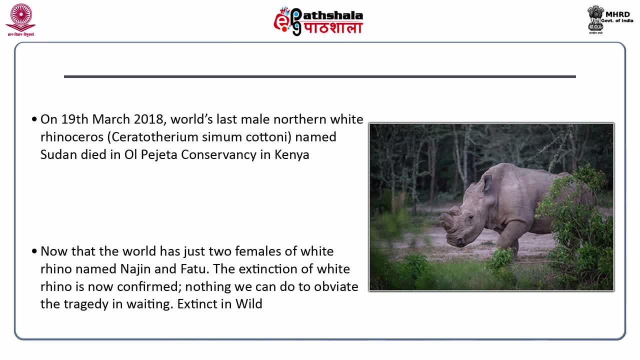 So now that the world has just two females of white rhino named Najin and Fudu, So the extinction of the white rhino is now confirmed. Nothing we can do to obviate the tragedy. in waiting, So it is: it's extinct in the wild. 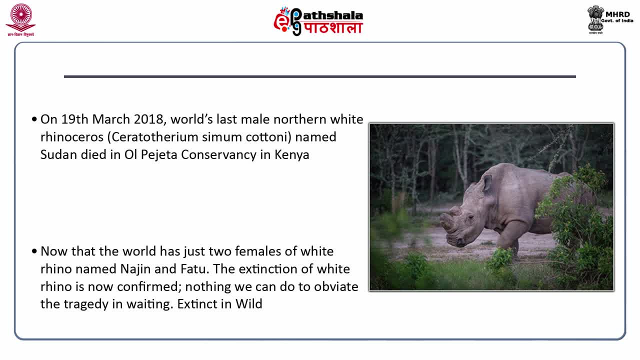 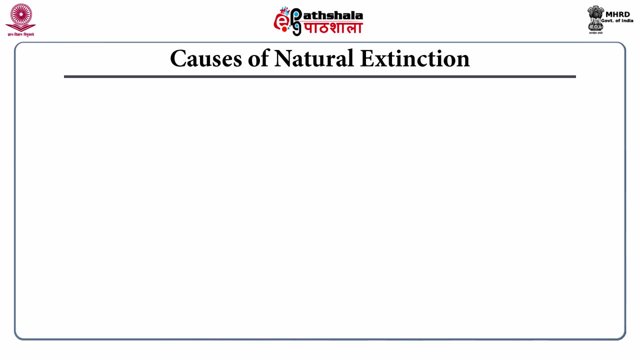 So we have only two female. So, of course, you know, regeneration from these two female is next to impossible unless we do some in vitro fertilization as well, as you know the cloning, of course, of course. So what causes these natural extinction? 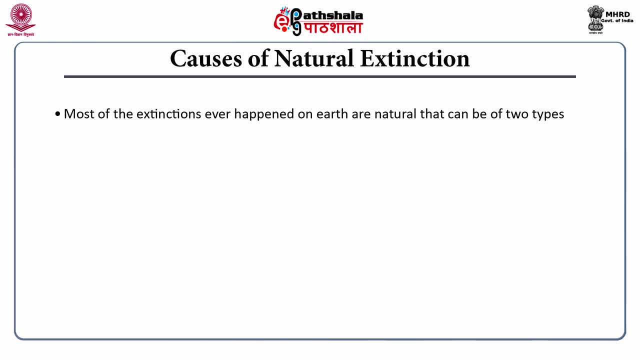 Most of these extinctions ever happened in the planet Earth are natural, and that can be of two types. So natural background extinction and mass extinction events. So natural background is ongoing extinction event every single day of the last four billion years, While mass extinction event is. 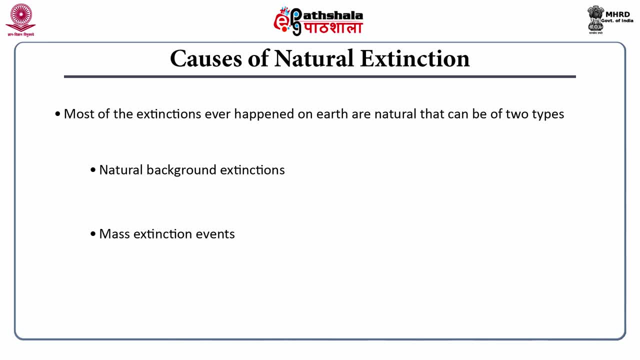 you know, extremely rare. but this is very, very important because that actually kills almost the entire diversity of plants and animals on the Earth, including marine and terrestrial flora and fauna. Causes of these natural background extinctions are multifaceted and often unknown. 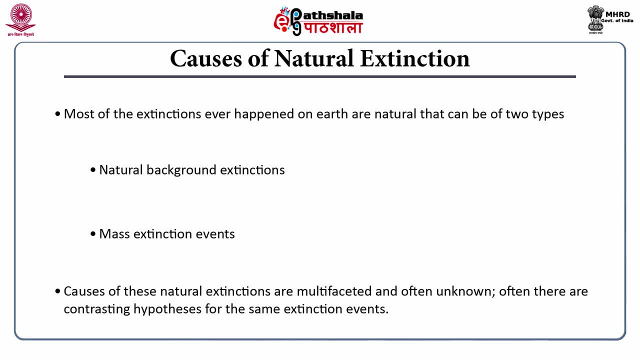 For example, it is analogous to the causes you know of a forensics expert. That is, actually they are the forensics expert, They are looking at the causes of a person, a dead person. So during the post-mortem, 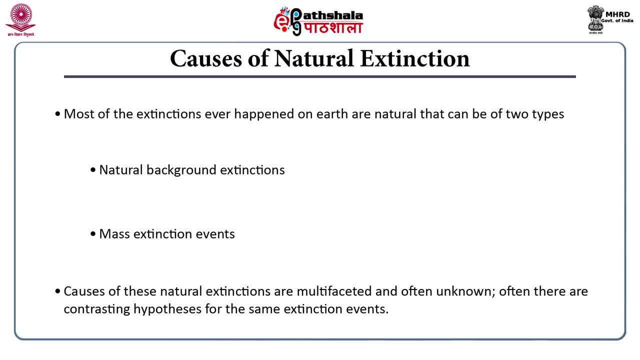 so that we can only reason With a certain number of probability for the possible reasons. So you can never confirm what really caused a species to go extinct, like an individual to go die or murder. So often there are contrasting hypothesis for the same extinction events. 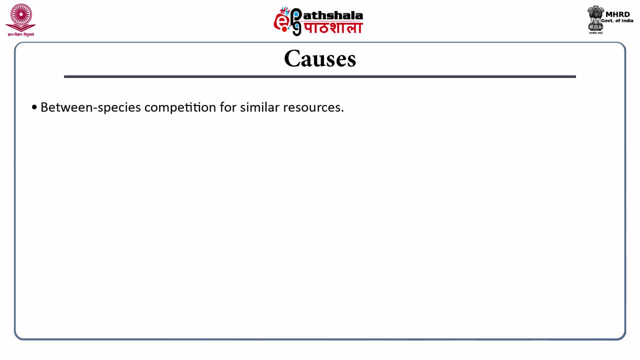 So ecological or climatological or geological are major factors, that is, the causes, causative factors for the natural background extinction. So in ecology, between species competition is one of the major driving factor for the similar resources. So resource utilization, competition between different species. 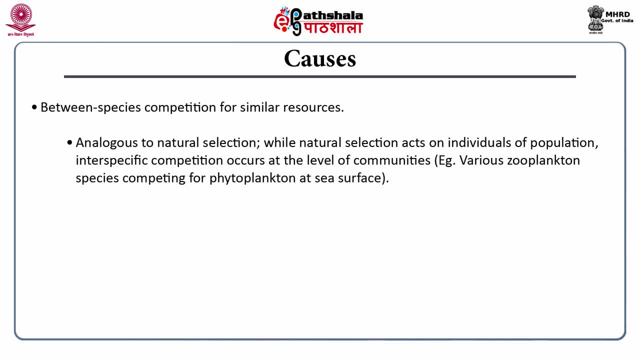 which is quite analogous to the natural selection. But in the case of natural selection that happens within a species, So mostly it's between the population, right, The natural selection happens at individual level of the population, But in this case it is between species inside a community. 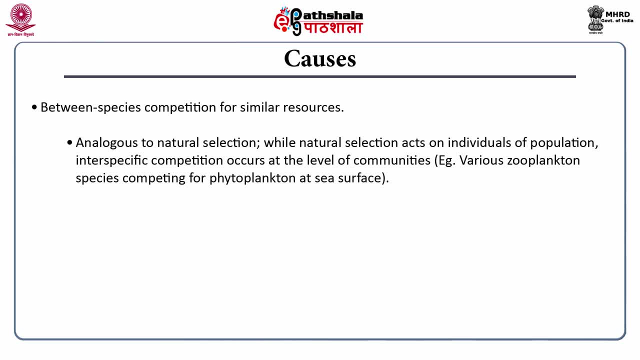 So, while natural selection acts on the individuals of a population, intraspecific competition occurs at the level of the community. One example would be various zooplankton species competing for the phytoplankton on the sea surface. So species can also lose its competitive advantage. 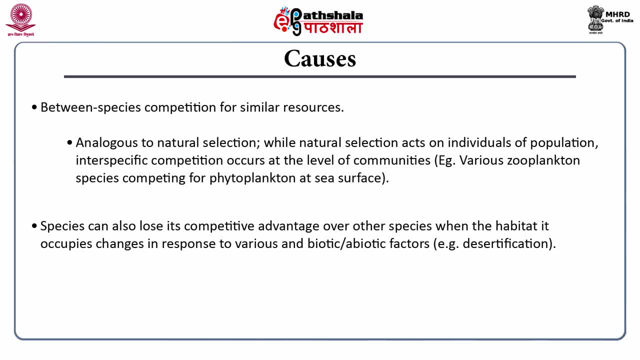 over other species when the habitat it occupies changes in response to various biotic or abiotic factors, For example desertification. So when an area becomes a desert, so associated changes on flora and fauna will drive a number of species to go extinct. 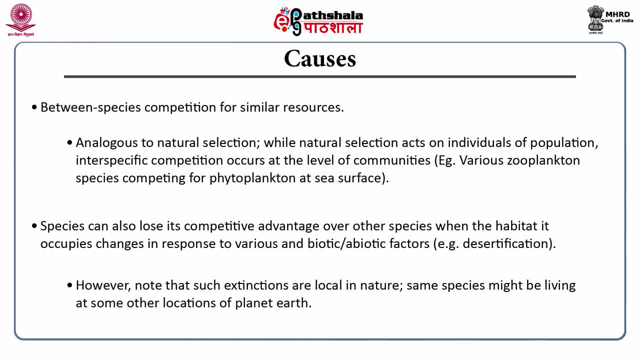 So, however, you should note that such extinctions are local in nature. Some species might be living at some other locations of the planet Earth. And how much is a species distribution, or the range, how big is the species range, is an important determinant. 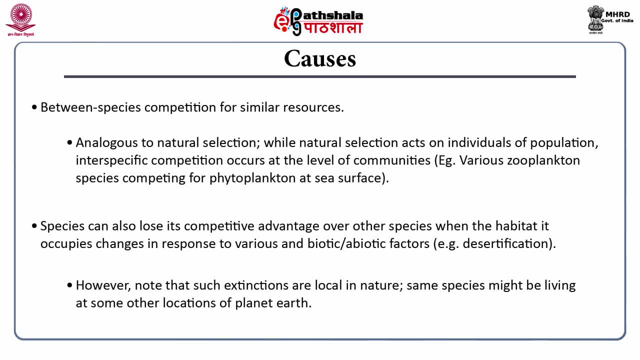 Will the species be survived in the case of an extinction event? For example, certain number of insects, members of insects. One example would be tardigrades, whose species range is extremely vast. The tardigrades you can find in space. you can find even underneath the ocean. So it is very, very difficult for the tardigrade species to go extinct. But you know, you can contrast that with the frog species. The amphibians are mostly endemic, So they are restricted to a particular location. So for the frog species to go extinct. 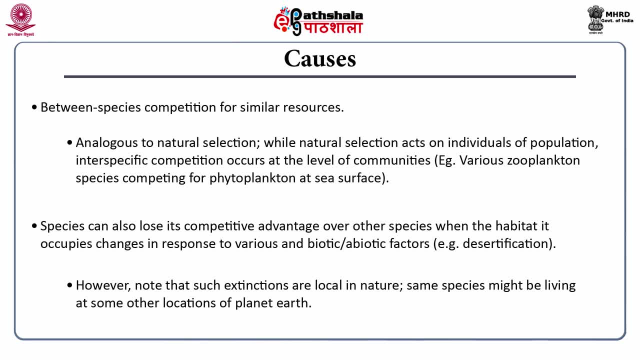 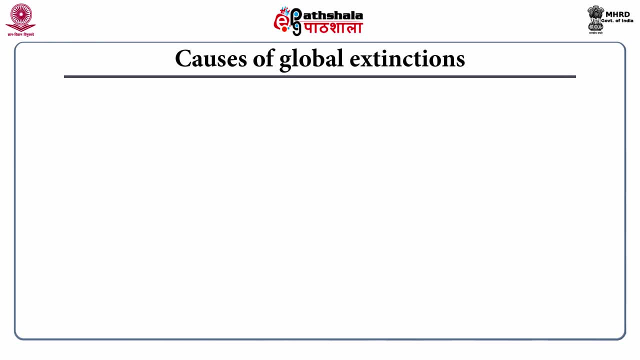 is a lot more easier Comparing with that of the tardigrade because of the species range. What causes the global- you know- massive extinction events? So there are several number of causes. So you can never say that all these five mass extinction events, 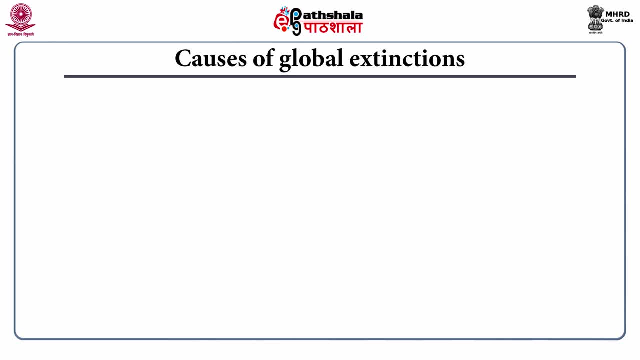 were caused by just one factor. That is impossible. So there are multiple factors and it's more often multi-faceted. So natural catastrophes could be one major reason. One reason could be asteroid impact or high UV rays Or infrared radiation. 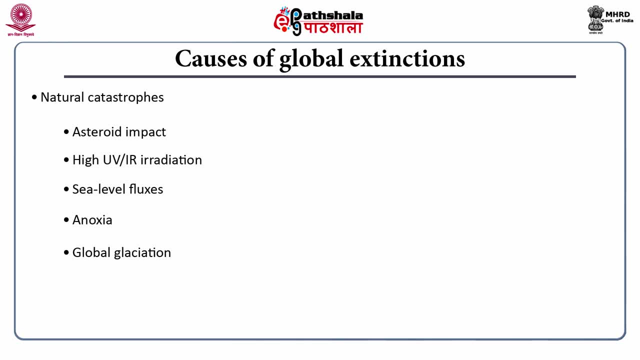 And sea level fluxes, Anoxia, Global glaciation, Volcanisms And many of these factors could be the causative agent of the next factor. For example, asteroid impact would cause massive UV radiation, while the asteroid is actually impacting on a particular place on the Earth's surface. 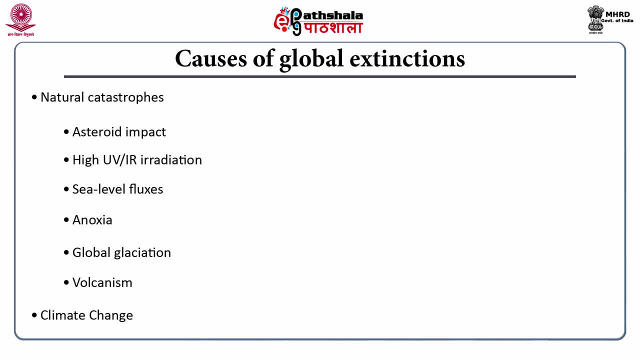 And after the impact, the dust will be spewed all over the atmosphere. That will cause, you know, nuclear winter. That will lead to global glaciation, The cooling down, So the global glaciation would cause the sea level fluxes. 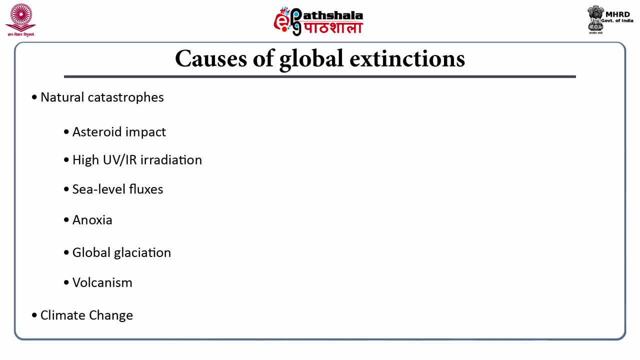 You know, while global warming will cause the rise of sea level, glaciation will cause the dip in the sea level. So all these are interconnected, So as the climate change The five major extinction events that have ever happened on the planet Earth. 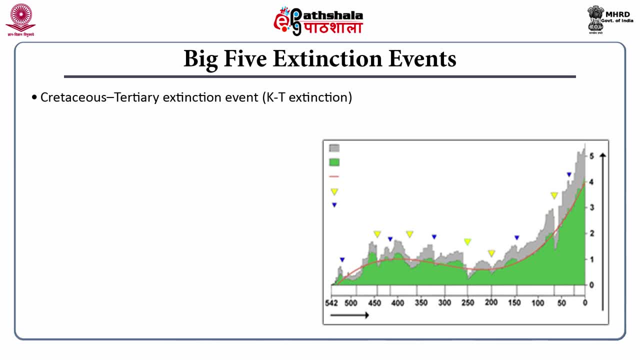 So these major five extinction events are: the Cretaceous Tertiary Event, also called KT Extinction, or Cretaceous Paleogene Extinction Event, which is the most recent one, Triassic Jurassic Extinction Event, Permian Triassic Extinction Event. 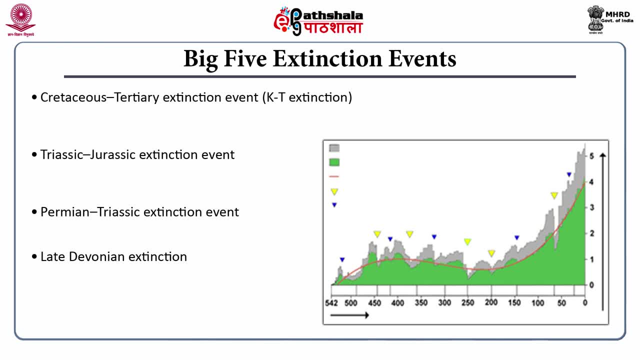 Late Devonian Extinction Event And probably the first one is Ordovician Silurian Extinction Event. So we will come to across all these major five extinction events, the causative factors of this, So mass extinction events, What are these? 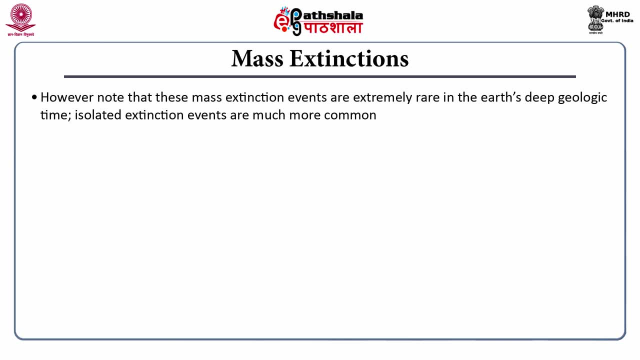 You should note that these mass extinction events are extremely rare in Earth's deep geologic time. Isolated extinction events are much more common. So local extinction events are a lot more common. Background extinction events might have caused a lot more, you know. 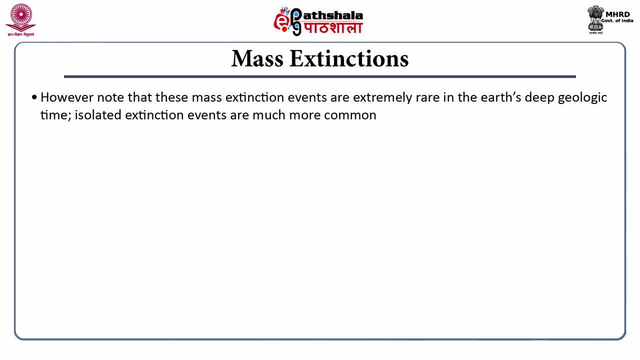 number of species extinction rather than the mass extinction events. But yet mass extinction events are very interesting because it caused, you know, extinction of a lot of species and mass. almost more than 70% of all species will go in one go. 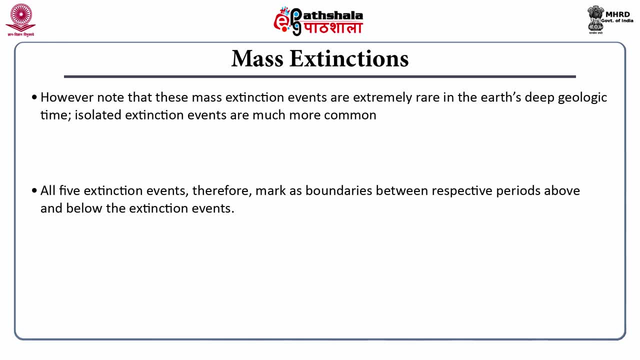 So all five extinction events therefore mark as the boundaries between the respective periods above and below of the extinction events. So most of these extinction events are marked in the rock layers. You know one above and one below, So you can see a drastic difference between the layers. 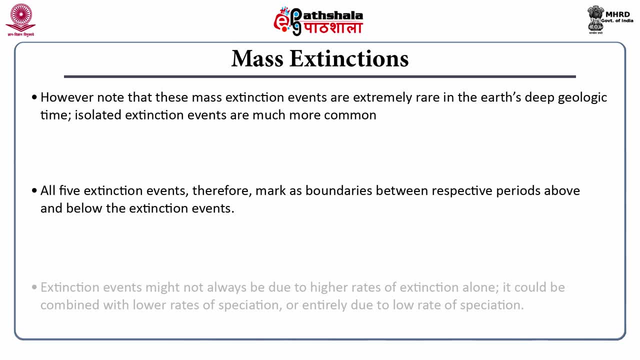 over the extinction events. So extinction events might not always be due to the higher rates of extinctions alone. So let the name of the event, let the name extinction event not be confusing to you. It could also be due to the fact that the speciation 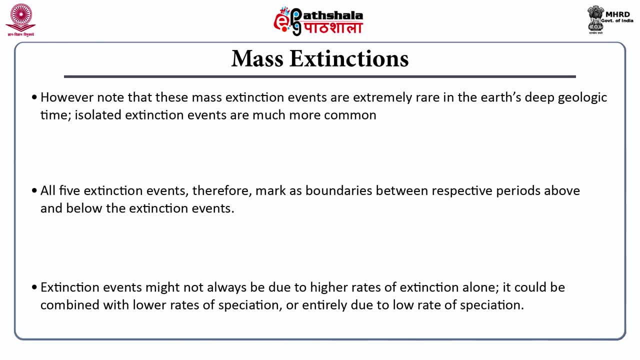 rate of speciation is very low. So either rate of extinction is very high or rate of speciation should be very low. So either way it will lead to a decrease in the global biodiversity. So it could be entirely due to the low rate of speciation. 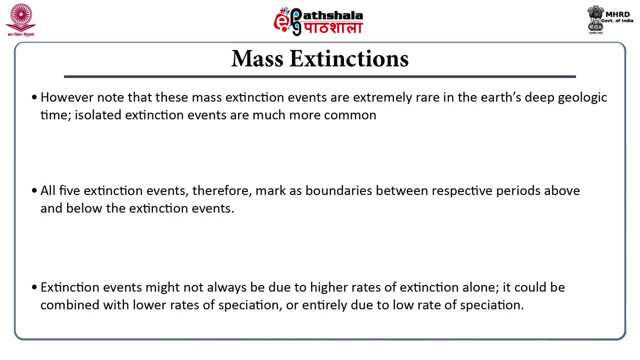 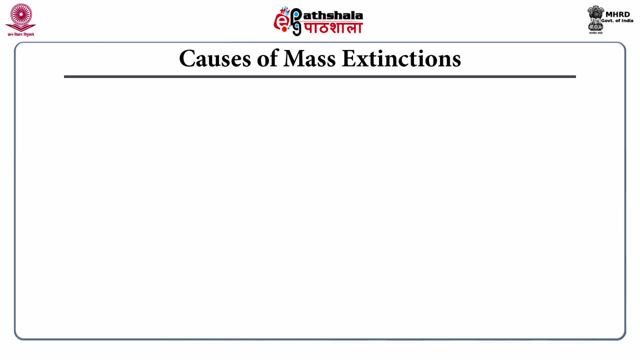 that we will see. one of the global extinction events was due to the low rate of speciation, not really because of the high rate of extinction. So we will see that exact causes of the different mass extinction events. So, while the exact initial causes are mostly debated, 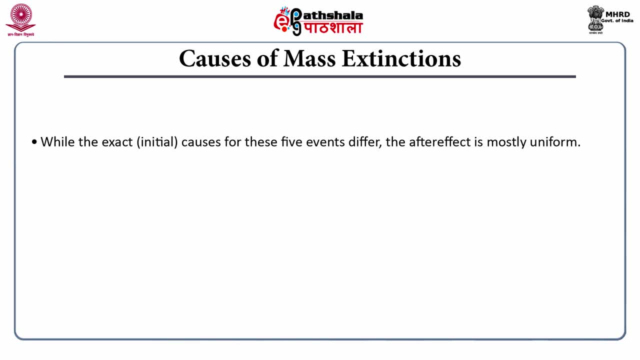 except in the case of the last extinction event, that is KPA, that is Cretaceous Paleogene, all the four. the initial cause is still debated. The after effect is almost uniform, So fluctuations in the global climate and the sea levels. 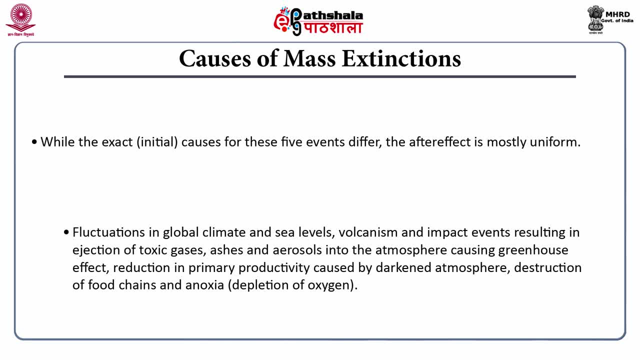 volcanisms and impact events resulting in ejection of the toxic gases, ashes, aerosols in the atmosphere, causing the greenhouse effect, reduction in the primary productivity caused by the darkened atmosphere, destruction of the food chains and anoxia, which is depletion of the oxygen. 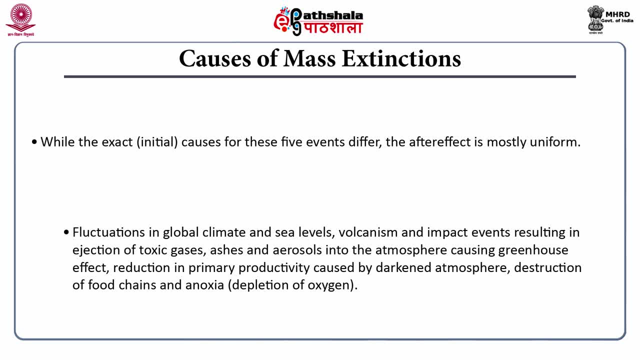 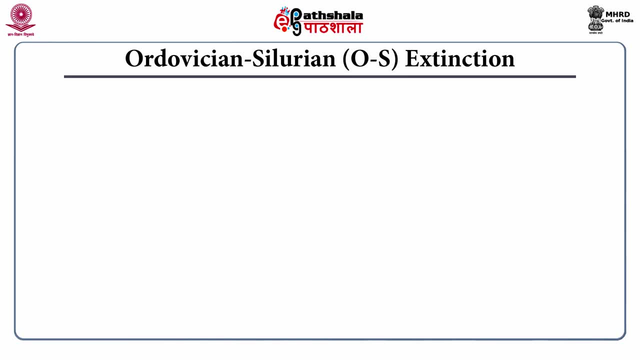 So all these are after effects of the initial event that drives the mass extinction event. The first one is Ordovician-Celurian extinction event. that is also called OS, the abbreviation which happened around 450 million years ago, which is the second most devastating. 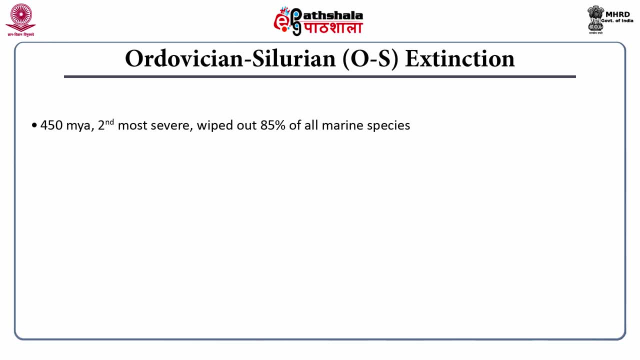 most severe extinction event, which has wiped out almost 85% of all marine species. So the cause is thought to be massive glaciation, the most severe glaciation in the current eon of Phanerozoic. This happened in Phanerozoic, of course. 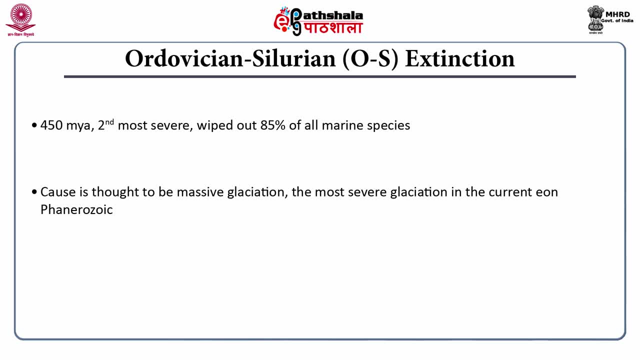 and this is the most severe glaciation, where almost the entire surface of the Earth was glaciated during the event of the Ordovician-Celurian extinction event. So during the glaciation, sea levels drop, as I just explained to you. 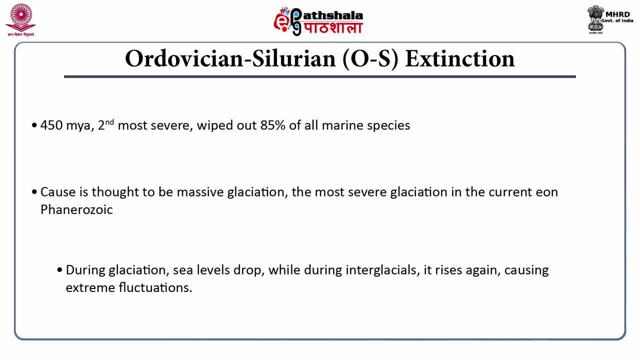 During the glaciation sea levels drop, while during interglacial, the relative warm period, sea levels rise. Right now the sea level is rising because right now it is interglacial. So next glacial time, glacial cycle: the glacial maxima. 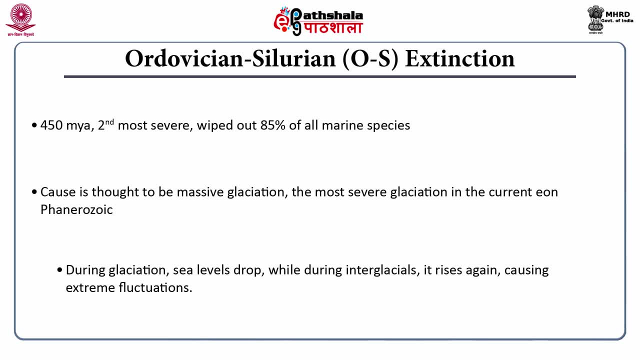 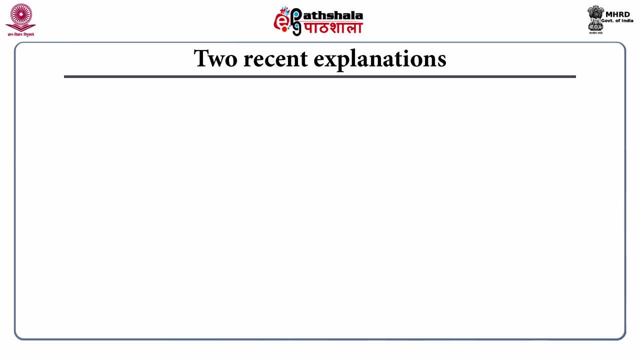 the sea levels will start sinking once again, So it will lead to extreme fluctuations in the global sea level. So what explains the Celurian-Ordovician extinction event? There are two explanations. The first explanation, I told you: the glaciation. 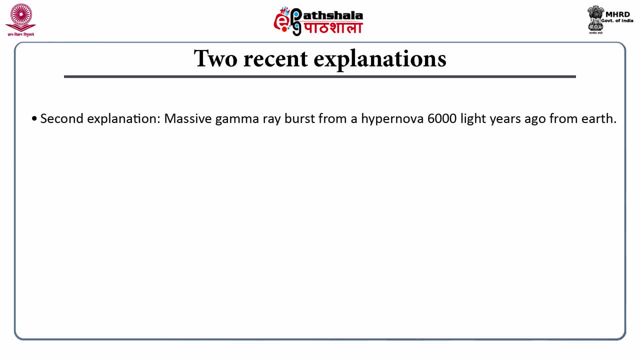 The second one is the massive gamma ray burst from a hypernovae 6,000 light years ago from the Earth. So that's even you know, 6,000 light years is such an immense distance. So light years is as you know. 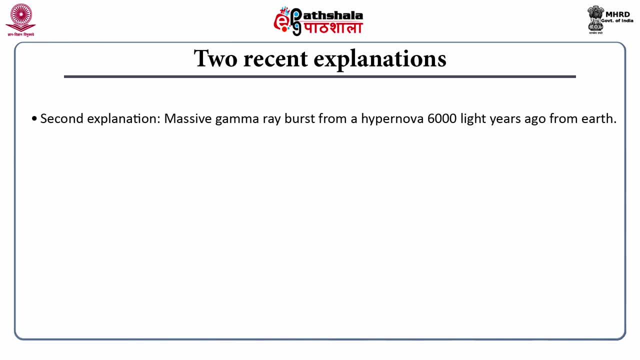 it's a measure of the distance. So how long will it take, How you know, for the light to travel in one year. so the distance that the light takes to travel one year is one light year. So 6,000 light years is really really far away. 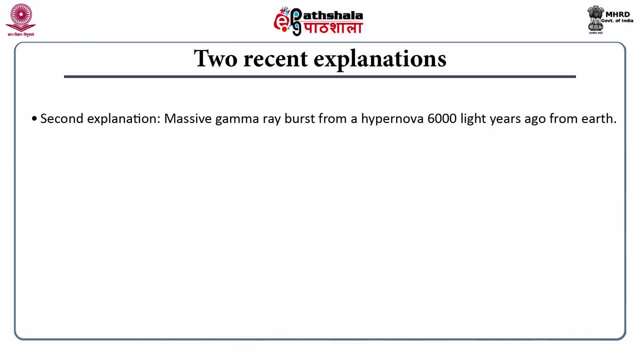 And even though the supernovae is quite far away, it's not merely supernovae, it's a hypernovae extreme, you know, extreme explosion of all these star dusts that might have caused a gamma ray outburst And even a 10-second gamma ray outburst. 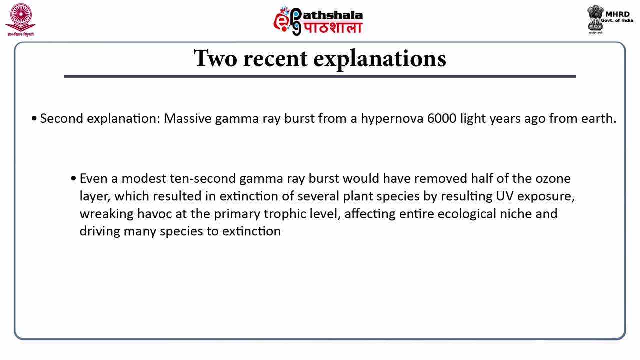 would have been removed half of the ozone layer. So that effect is a lot more serious, because without ozone layer none of the surface inhabitants on the planet Earth could ever live, So resulting several plant species and will go extinct almost immediately, And you know. 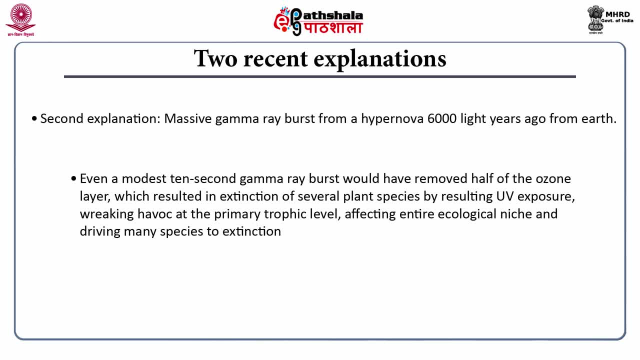 the resulting UV exposure. because of absence of the ozone layer, the UV exposure, the radiation, will be quite high. That would have wreaked havoc at the primary trophic level, So affecting the entire ecological niche and driving many species to extinction. And now we have a third. 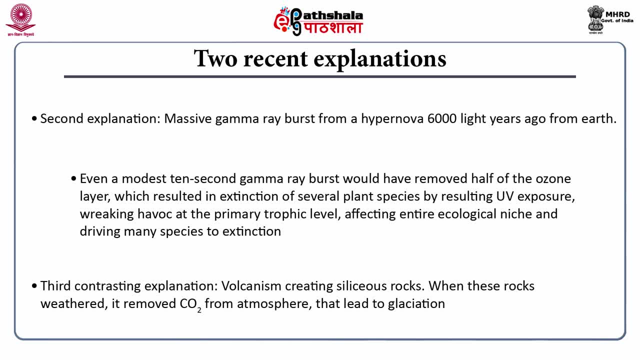 the contrasting explanation for the same Silovian-Odovician extinction event is a volcanism creating siliceous rocks all around the world. When these rocks weathered, it removed the CO2 from the atmosphere that led to the glaciation. So that's a very interesting explanation. 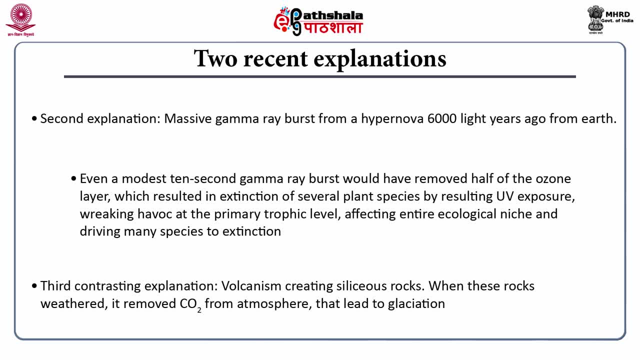 you know, the particularity of the siliceous rock is that when the siliceous rock weathers, so it actually removes the CO2.. It absorbs the CO2 because siliceous combine with the carbon to form a silicate rock. 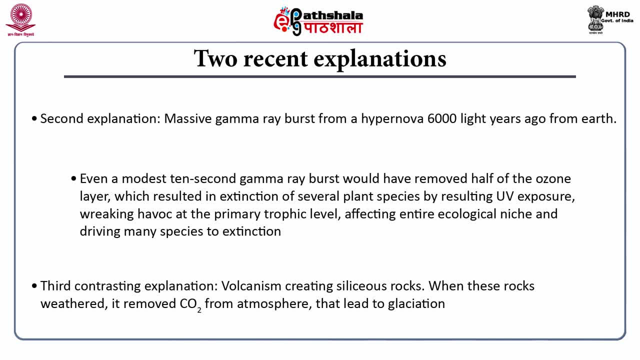 you know the rock, So its sequester. it removes the carbon dioxide from the atmosphere, as the CO2 is a greenhouse gas. More and more CO2 is being removed from the atmosphere. that will result in the global cooling and, ultimately, a glaciation. 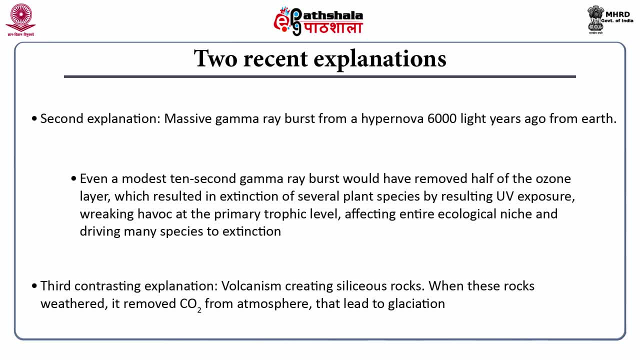 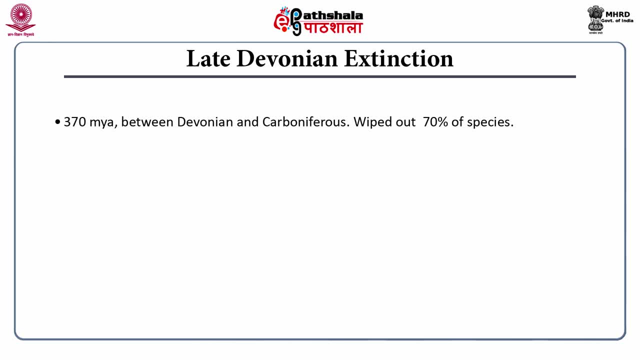 So probably that might have caused initial glaciation event. Second, in our extinction event is late Devonian extinction. that happened 370 million years ago between Devonian and Carboniferous eras, So it has wiped out almost 70% species In terms of extinction intensity. 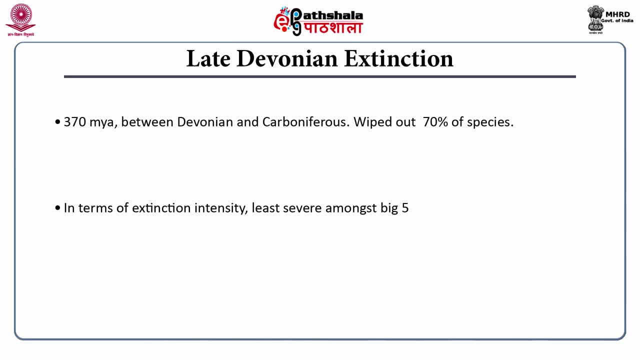 late Devonian extinction is the least severe amongst the big five. So the main trigger of this extinction event is the evolution of vascular plants in the Devonian. So whenever the vascular plants have evolved in the Devonian so that have actually consumed a lot more CO2 from the atmosphere, 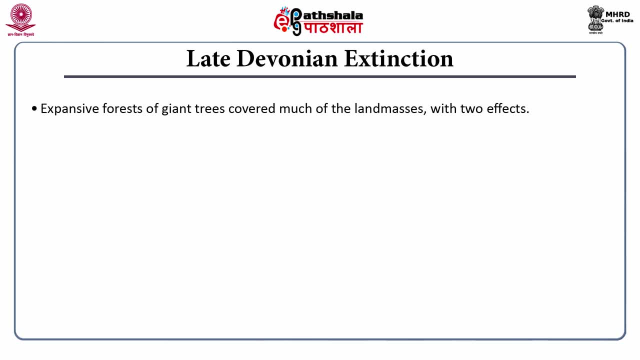 and that led to the global cooling. So, expansive forest of the giant trees covered much of the land masses during the Permian period. So, with the two effects, what are the effects of this expansive forest covering the earth? you know, during the Devonian period? 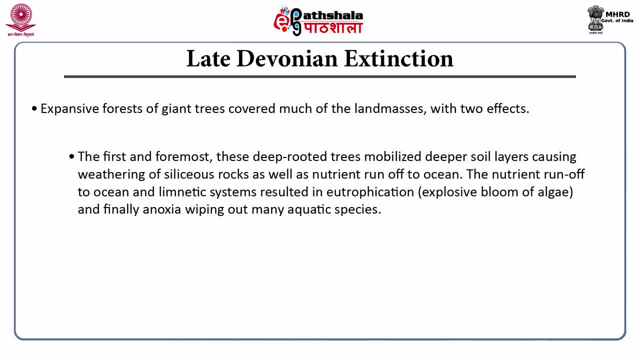 The first and foremost, these deep rooted trees mobilized deeper soil layers, causing the weathering of the siliceous rocks as well as the nutrient runoff to the ocean. So because the siliceous rocks weather, as I just explained to you, the siliceous rock weathering 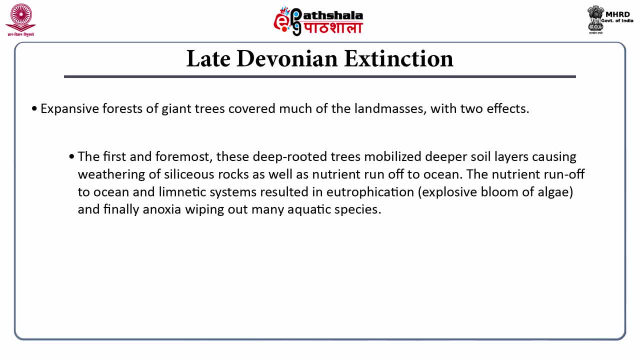 would cause CO2 sequestration. that would lead to the global glaciation. Now, nutrient runoff to the ocean would cause, you know, the nutrient load to increase in the oceanic habitat. That would lead to eutrophication, and eutrophication is nothing but. 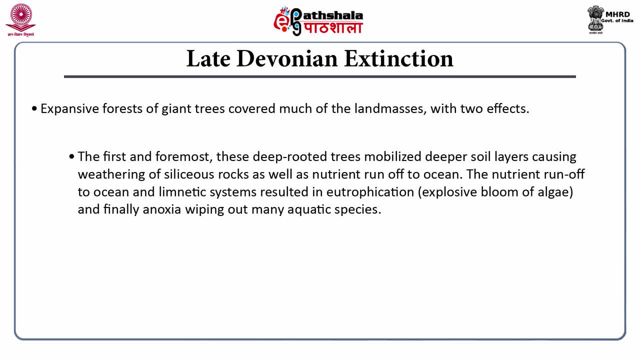 you know the oxygen consumption by the algal blooms. So that would lead to anoxia. Anoxia is very less dissolved oxygen levels on the global ocean, So finally that would asphyxiate the entire. you know the marine organisms. 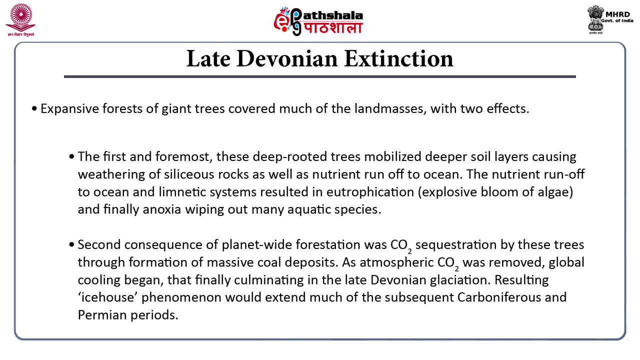 So that is the first level. Now, second consequence of the planet wide deforestation is CO2 sequestered by these trees through the formation of massive coal deposits, The CO2 direct sequestration by the trees of the Devonian era That might have actually led. 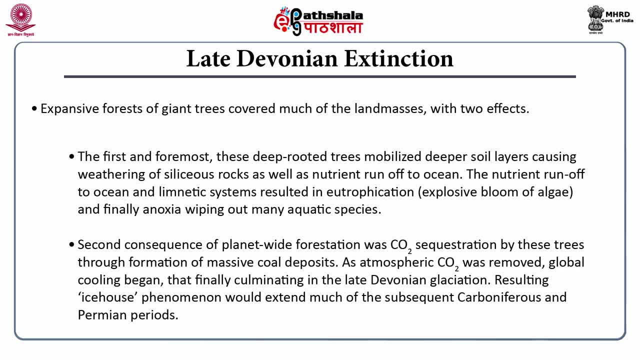 to a global glaciation. As atmospheric CO2 was removed, global cooling began and that finally culminating in the late Devonian glaciation, resulting in the ice house phenomenon that would extend much of the subsequent carboniferous and Permian periods. Next is Permian extinction event. 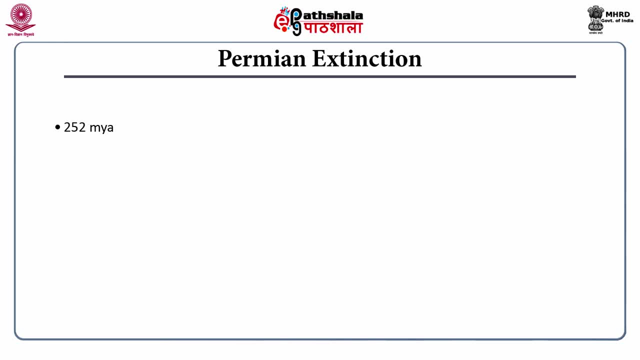 that happened 252 million years ago and in terms of extinction impact or intensity, Permian is the biggest one. You know it's also called the big dying event, So it drove the extinction of 96% of the all marine species. So it is like the complete devastation. 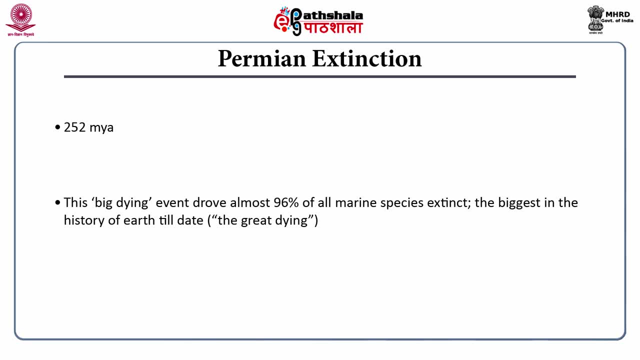 So that is the biggest extinction event in the history of the life on planet Earth. There are several contrasting explanations for the cause, yet there is no consensus exist. Recent research have led to a kind of consensus about what really caused the Permian extinction. 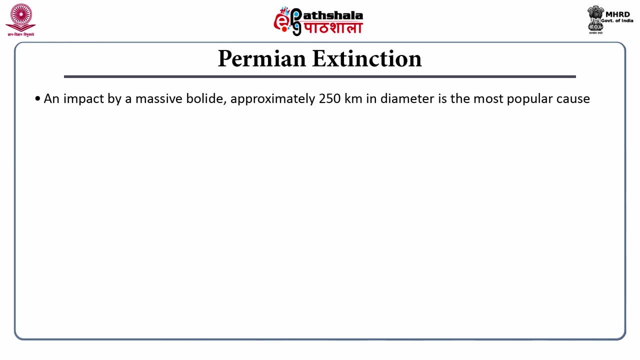 The consensus is that there is a giant impact by a massive bolide asteroid, approximately 250 km in diameter, the biggest asteroid impact ever that the Earth has witnessed. That is the most popular cause Now, an indirect coexistence of such an impact crater. 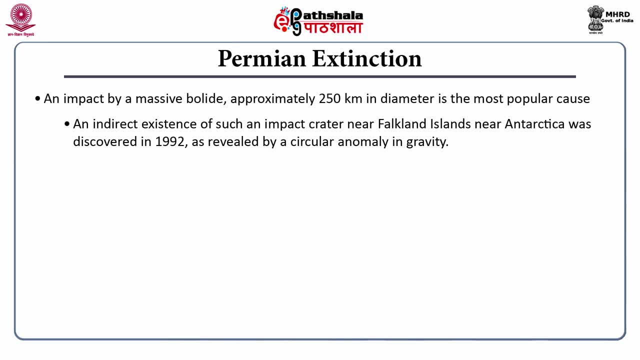 near Falkland Islands, near Antarctica, was discovered in 1992.. So such a crater, the indirect fluctuations in the magnetic activity, So it was. it has been published in 1992 as revealed by a circular anomaly in the gravity The impact might have triggered. 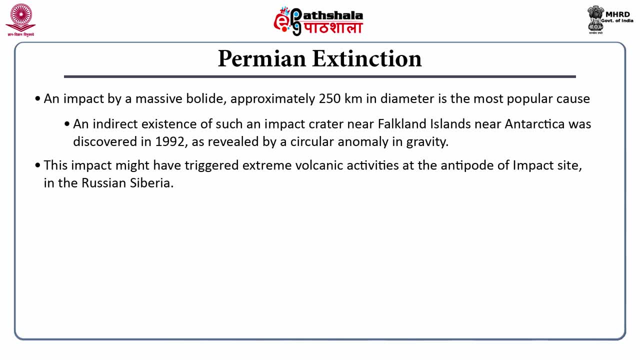 extreme volcanic activities at the antipode of the impact site. So it is near Antarctica, that is near South Pole. So the antipode of that impact crater is in the north, So near the North Pole, in the Russian Siberia it might have actually. 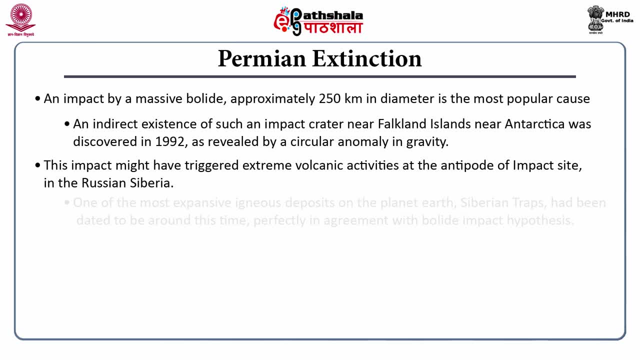 you know, caused volcanic eruptions, One of the most expansive, igneous. you know the deposit on the planet Earth Siberian traps had been dated to be around this time, perfectly in agreement with the bolide impact hypothesis. So extreme volcanism at Siberia. 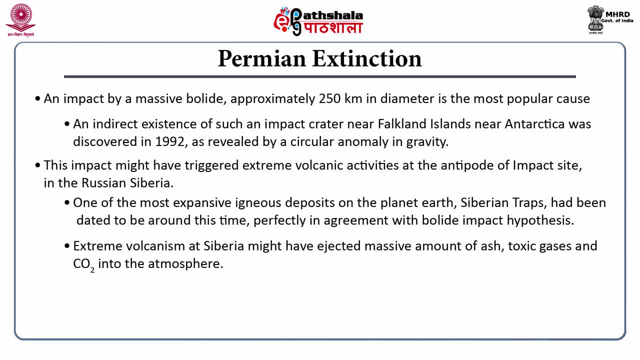 might have ejected massive amount of ash, toxic gas and carbon dioxide into the atmosphere. that might have actually formed a kind of layer that might have blocked the sun rays to come inside. So it might have triggered a nuclear summer and subsequently the entire Earth might have actually glaciated. 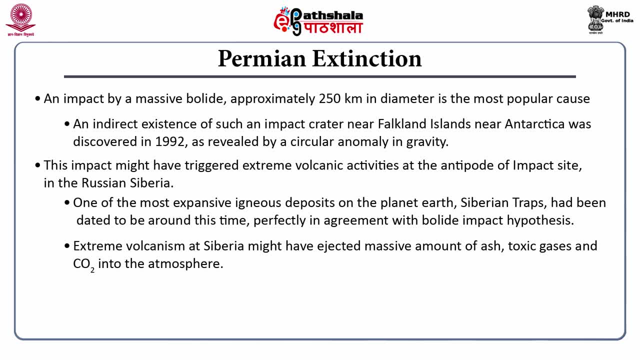 So all these are the chain of events that might have triggered by the initial bolide impact. So it also caused the ignition of massive cod beds that resulted in further rise in oxygen levels and more atmospheric ash. The dense ash layer might have completely blocked out. 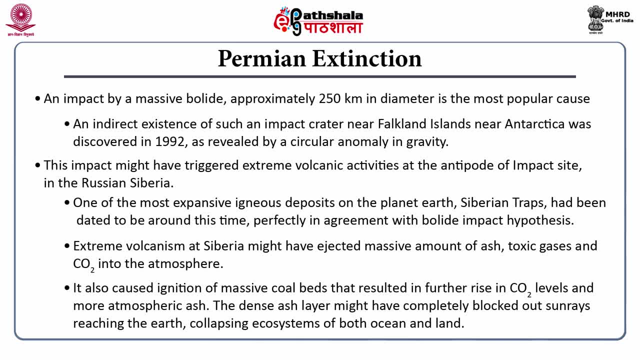 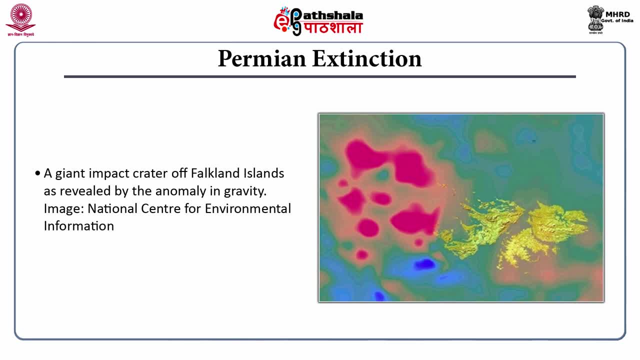 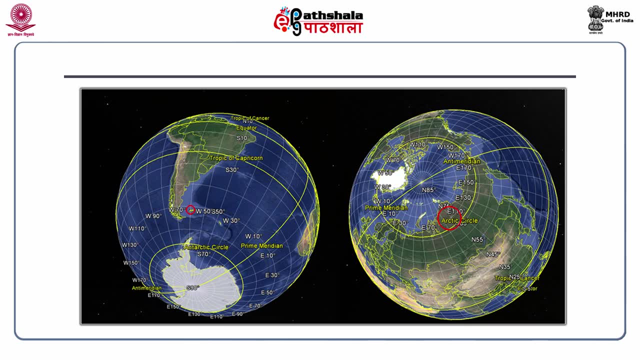 the rays reaching the Earth, collapsing the ecosystems of both ocean and the land. So the Permian extension event: the impact crater was off the Falkland Islands, as revealed by an anomaly in the gravity. So why does most of this impact happen in the ocean? 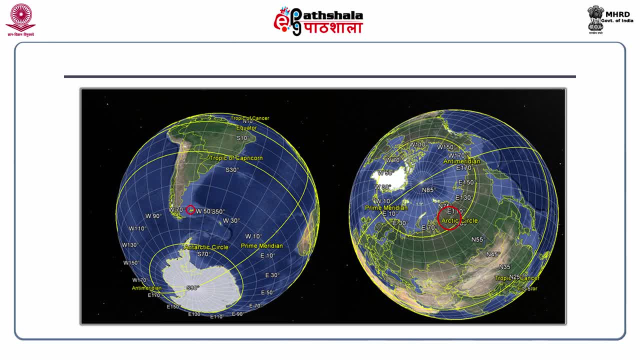 Because the Earth is almost ocean right. 71% of the Earth's surface is 71% of the surface of the Earth is ocean. So chances are very high that you know, a stochastic impact of an asteroid would happen in the ocean. 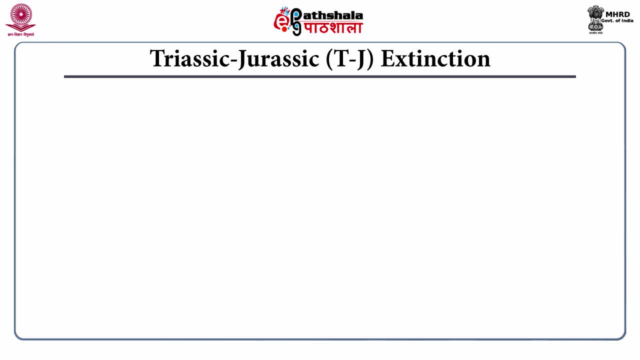 rather than on the land. Next extension event is Triassic-Jurassic extension. that happened near the beginning of Jurassic, so end of Triassic almost 200 million years ago. So it wiped out 70 to 75% of the all species on the Earth. 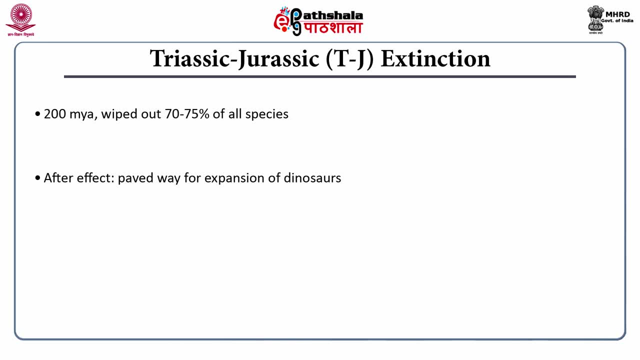 What are the aftereffects of this? It paved way for the expansion of the dinosaurs, So previous, you know, sauropsid mammals, so the reptiles, they actually out-competed by the dinosaur because the competent of those dinosaurs actually went extinct. 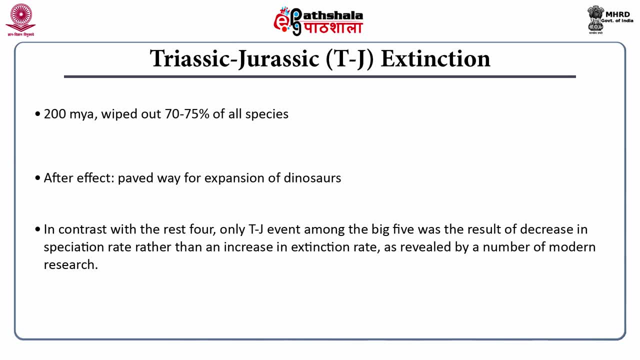 during this particular extinction event. So, in contrast with the rest of the four extinction events, only TEJ event among the big five was the result of the decrease in speciation rate, because the background extinction rate remained the same, Only the speciation rate went down. 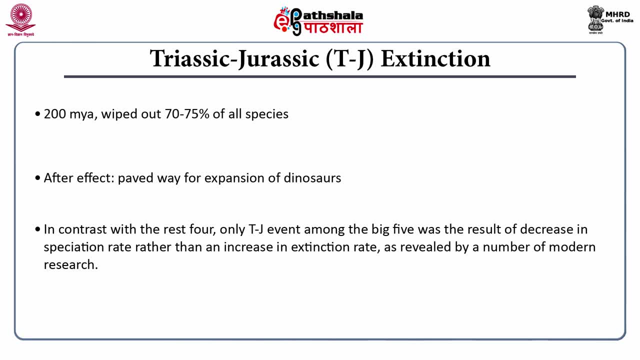 So, as revealed by a number of modern scientific research. so background extinction rate remained the same, but the speciation. what actually drives the speciation rate to go down? So there might be various mechanisms. So, amongst the contrasting hypotheses, the gradual climate change. 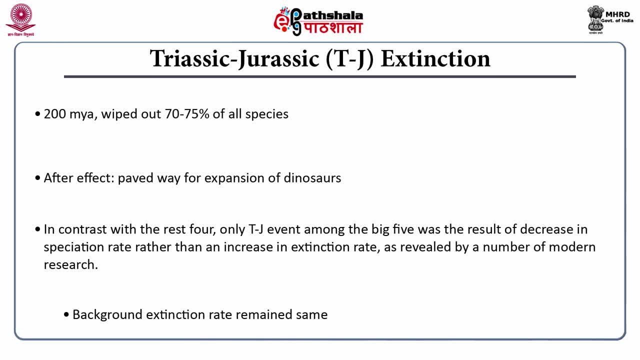 hypothesis, along with the ocean acidification. so exactly same thing as of today. So today the world is suffering from the global warming and also by the ocean acidification, as you see, because of the greenhouse effect, because of the extreme CO2 levels, as well as the methane levels. 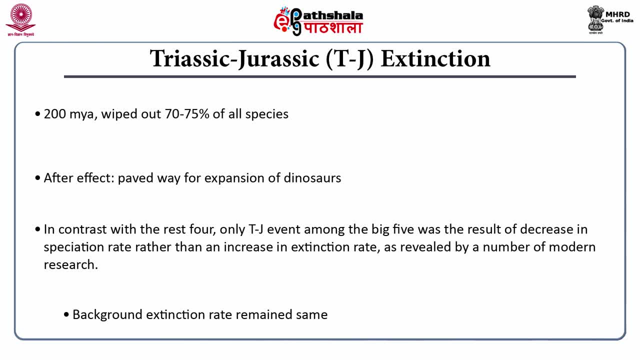 in the atmosphere, CO2 mixed with the oceanic water and the marine water, the seawater, the pH of the seawater goes down. So the acidification happens because of the carbonic acid formation, right, So all these are slow process. 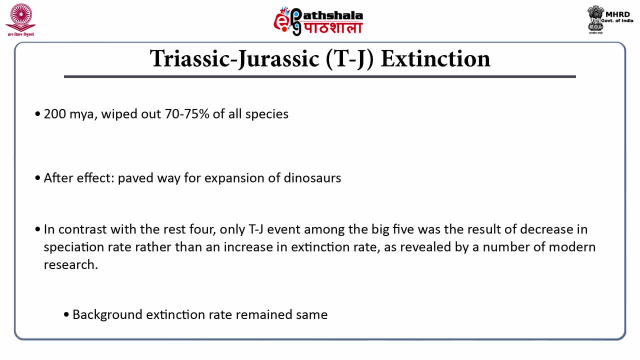 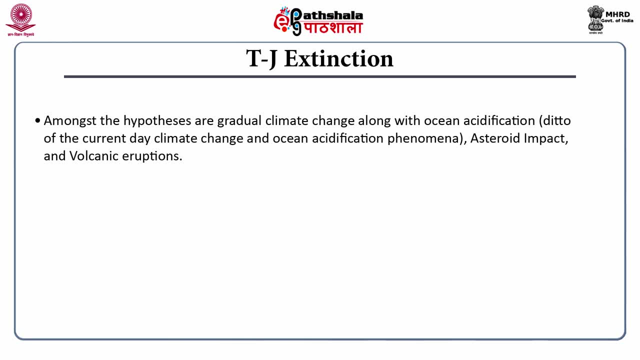 So this exactly same climate change might have triggered the T-J extinction event as well. So asteroid impact and volcanic eruptions are contrasting hypotheses for the T-J extinction events. But in the case of asteroid impact or volcanic eruptions, anybody would sufficiently argue to see an increased 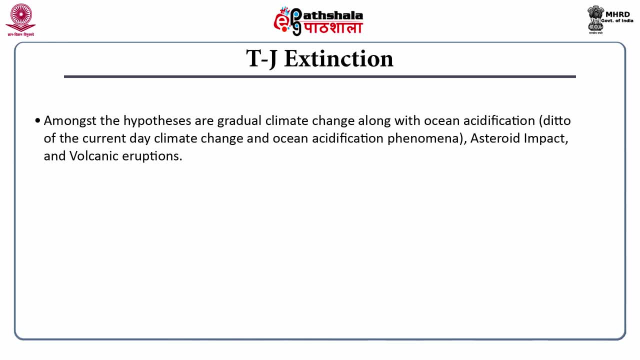 extinction event, But in this case extinction rate was not. actually no anomaly was observed in the case of extinction rates, but only that the rate of speciation went down. So a possibility that the series of volcanic eruptions initiated great changes in the global carbon cycle. 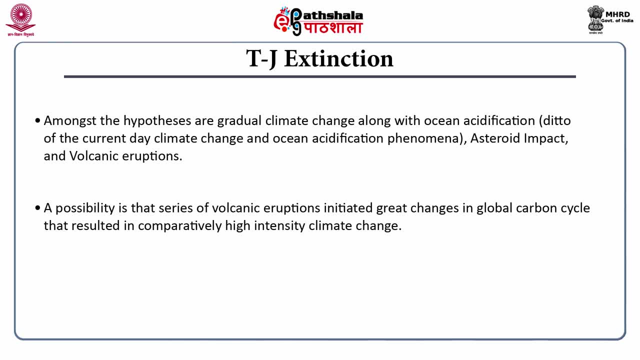 that resulted in comparatively high intensity climate change. An immediate aftermath of this extinction event is the breakup of the supercontinent Pangea. But you know, you should know, that the break of Pangea is not connected to the T-J extinction, So T-J extinction event. 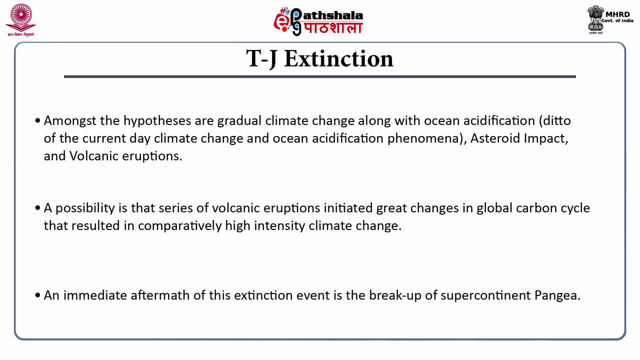 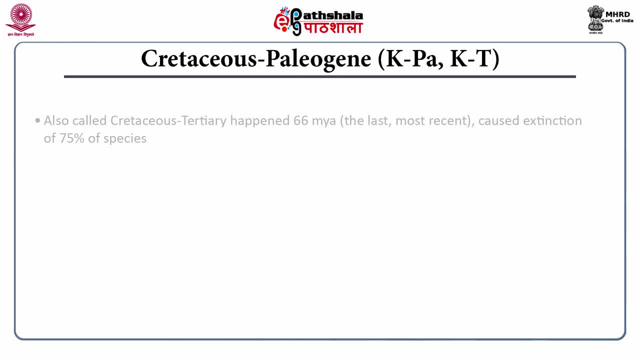 was not the cause of the breakup of the Pangea, So that is not related at all because it's an extinction event that's concerned with the global biodiversity. A major extinction event is the latest one that is called Cretaceous Paleogene. 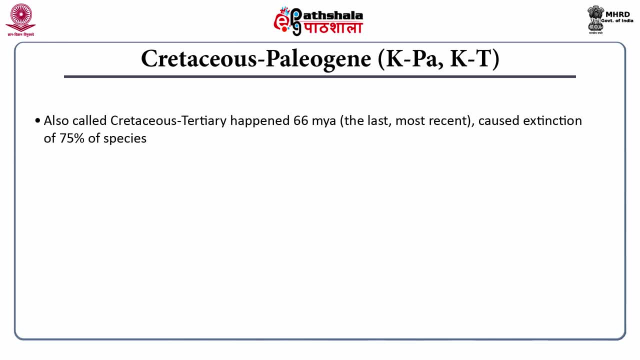 KPA also called KT, which is quite popularized by various movies as well as documentary. For example, you know the dinosaur movies and number of movies that came for the Jurassic Park or Jurassic World. The KT extinction event is prominently featured in these movies. 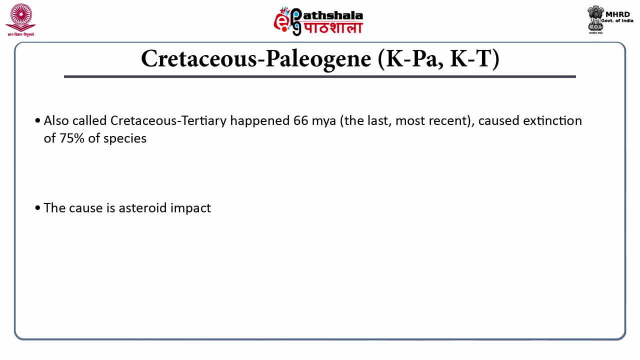 So the cause of this particular event is almost certain. There is a consensus that the cause is now considered to be thought to be the asteroid impact, a big asteroid that actually struck the Chicxulub location. The crater is called Chicxulub. 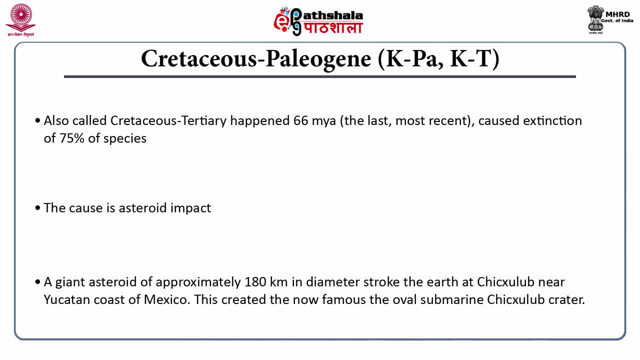 in the Yucatan coast of Mexico. So the asteroid might have been at least 180 kilometers in depth, in the diameter so, which is almost like the Permian one, but the Permian one was a little bit bigger: 250 diameter. 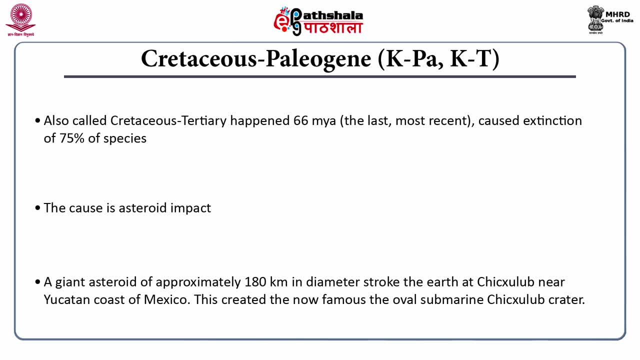 but this one is 180 kilometers in the diameter, which is immense, really immense. So this crater, the now famous Oval Submarine Chicxulub crater, as you can see in this picture, The key discovery of this particular impact hypothesis happened. 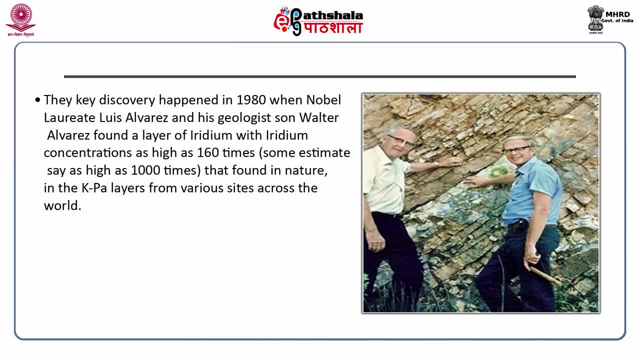 you know, in 1980 by the famous physicist, the American physicist Luis Alvarez, who was subsequently awarded with Nobel Prize for this discovery, along with his son, a geologist, Walter Alvarez, They found that the layer of iridium, in that particular 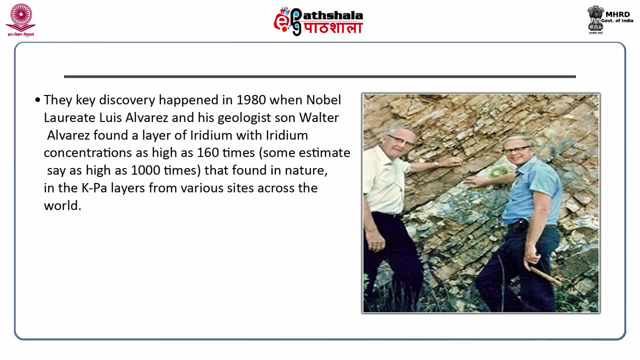 you know, rock formation around 66 million years back contained iridium. that is a rare earth element. So the concentration of iridium in that layer is 160 times that found in the nature in the earth. So it's highly unlikely. 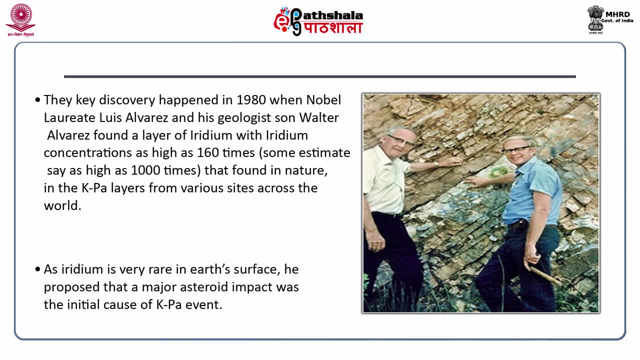 that this iridium came from earth. It might have came from, you know, an extraterrestrial source, that is, by the impact of this particular asteroid. So this is actually a beauty of working with geology. So the log layers are uniform. 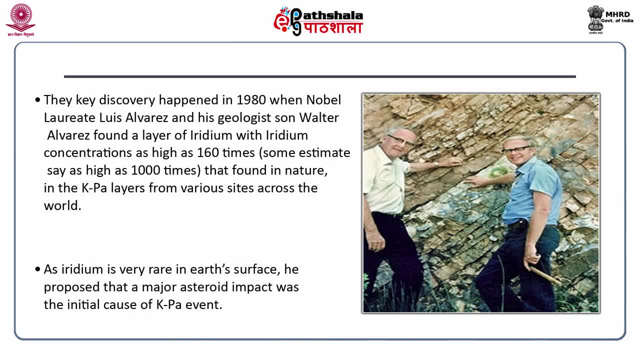 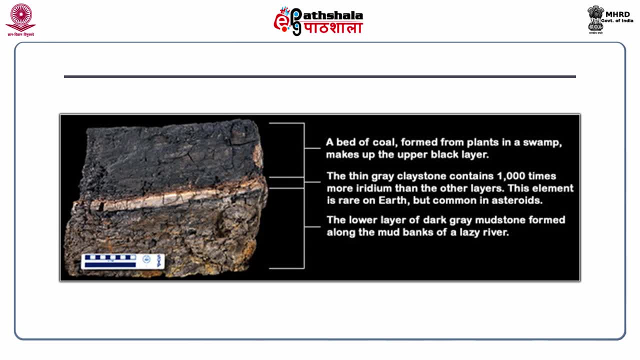 So, no matter where you sample- Japan or China or South America or South Africa- 66 million years old layer of this particular rock are all similar and all these layers contain, you know, this iridium. So that is actually a very good. 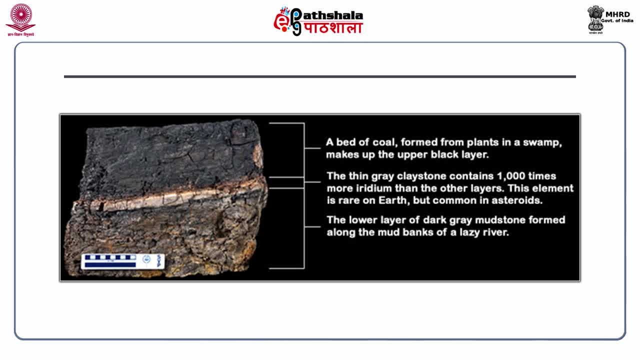 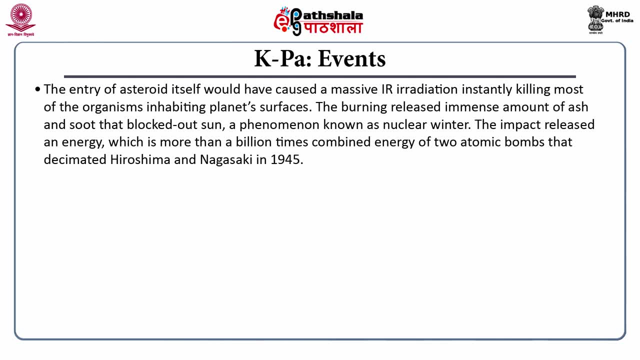 substantiating evidence for this particular hypothesis of KPA. So it might have triggered a series of events. One is that when this particular asteroid hit, so it might have caused a massive infrared irradiation instantly killing most of the surface dwelling organisms on the planet earth. 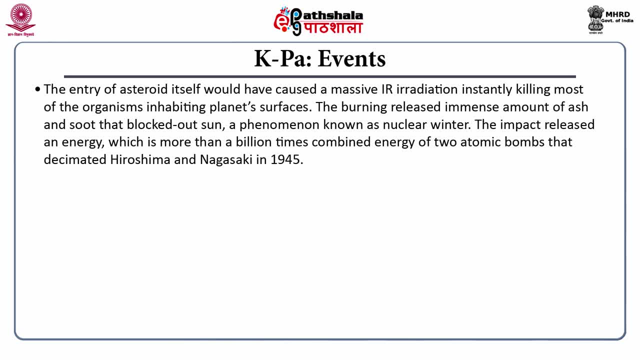 So the burning of released immense amount of ash and soot that blocked out the sun, a phenomenon known as the nuclear winter. So sun rays cannot actually come in it because of the ash layers. you know, a layer of ash actually prevents the incoming. 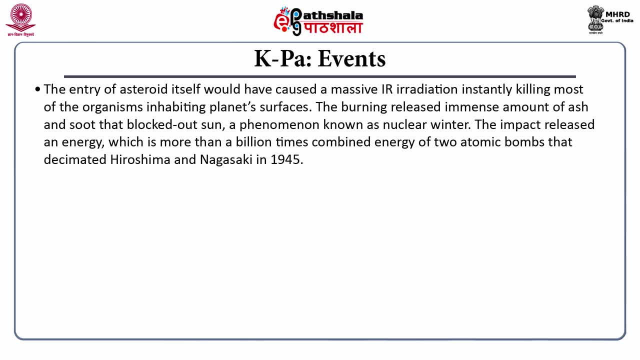 of the earth, So it might have drastically draw down the temperature of the planet earth. So glaciation happened it The impact site was rather rich in sulfur, So again that might have caused the sulfur. as you see, it will actually go to the sulfuric acid. 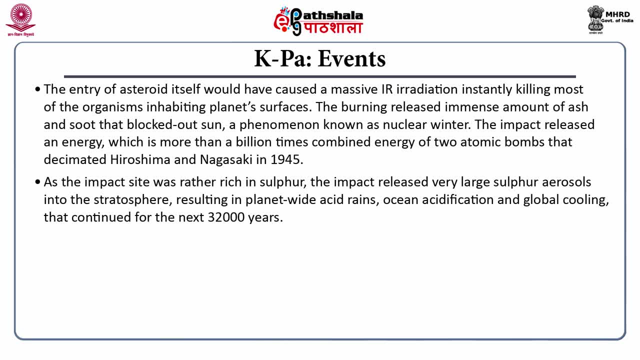 and acid rain might have actually happened. you know that it might have triggered acid rain, as well as the acidification, the global acidification, killing the phytoplankton. So killing the phytoplankton, reducing the oxygen level of the atmosphere. 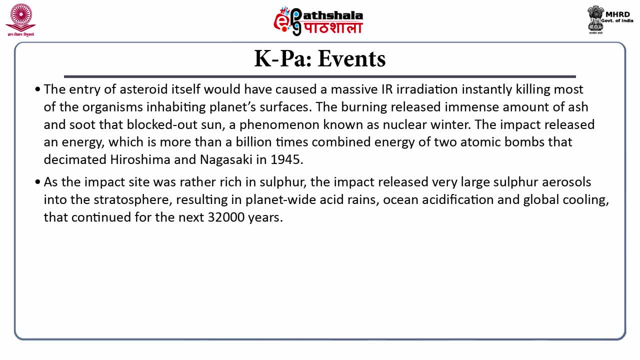 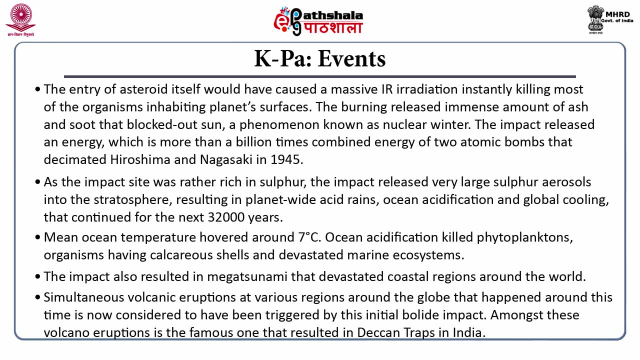 asphyxiating most of the aerobic organisms. So mean ocean temperature hovered around seven degrees Celsius throughout the world. See, it's quite cold. So it's all because of the global cooling that happened after this KT extinction event. Simultaneous volcanic eruptions. 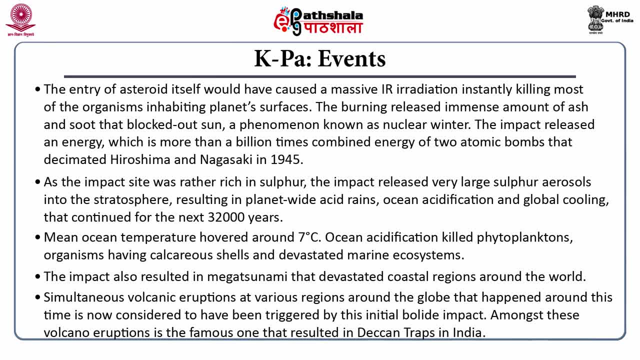 at various regions of the globe happened around this time is now considered to have been triggered by this initial blight impact. Amongst these is one that resulted in decantraps in India. So India have got decantraps Again. that decantraps. 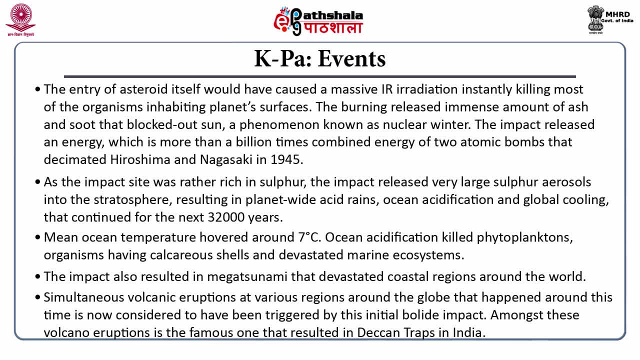 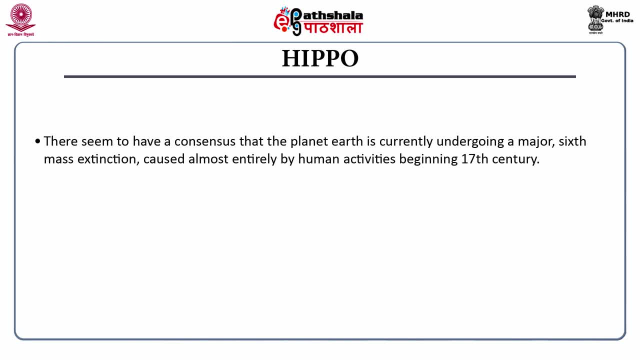 is dated around 66 million years or perfectly in agreement with this initial blight impact. Last extinction event is the acronym HIPPO, H-I-P-P-O, And there seems to have a consensus among the climatologists as well as the geologists. 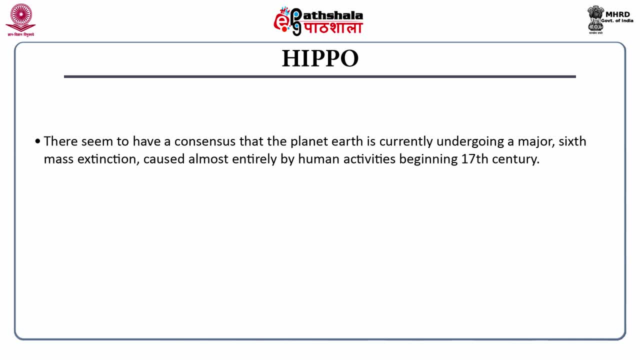 that the planet Earth is currently undergoing a major decontamination by the human activity. So this is totally anthropogenic. beginning in 17th century after the industrialization in UK Britain, HIPPO H-I-P-P-O is the sixth mass extinction. 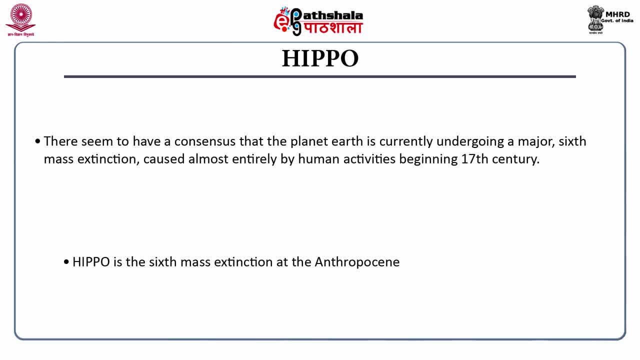 in the Holocene and now the boundary is almost confirmed- in around 17th century. Now this particular ion is called the Anthropocene, the latest period of the geologic history. Anthropocene because of the human being, So HIPPO, the acronym. 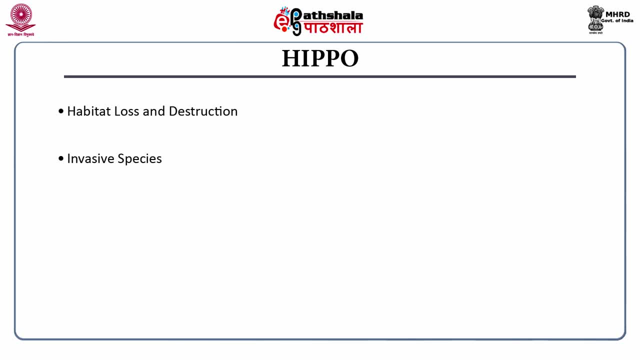 for the Anthropocene means destruction and destruction, the human mediated destruction, as well as conversion and loss of the habitat, for example, the wetlands. Invasive species: because of the interaction of the species by the exotic species that wreak havoc on the local region where it is. 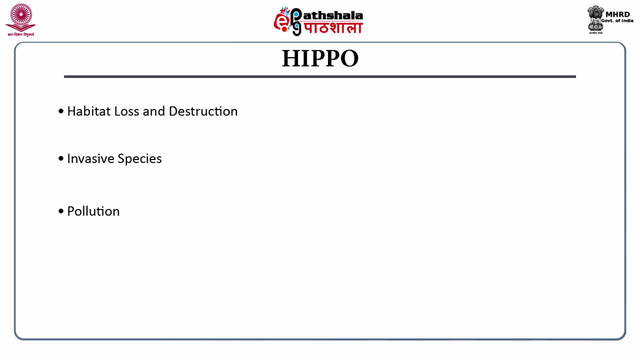 actually invaded into Pollution because of the human activity: tremendous number of species, human population- probably this is the root cause of the entire HIPPO phenomenon: the population expansion that is causing tremendous load on the atmosphere as well as the biodiversity, and, finally, over harvesting the resource. 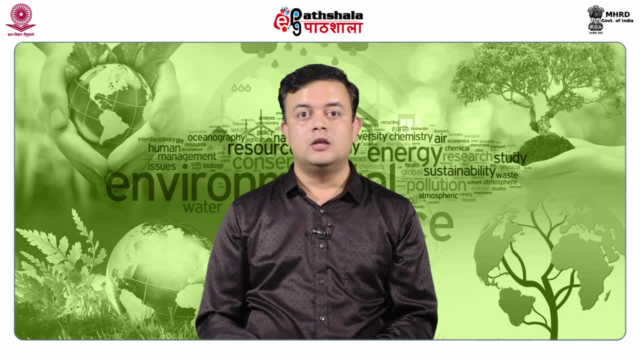 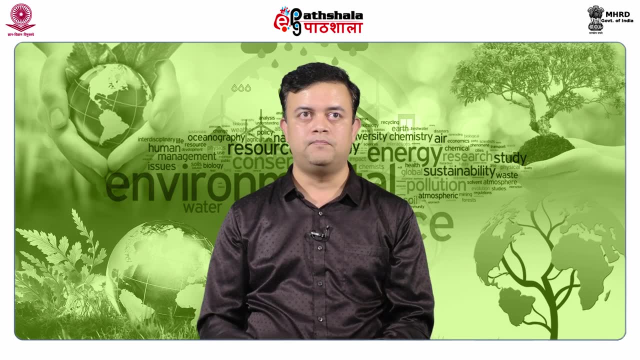 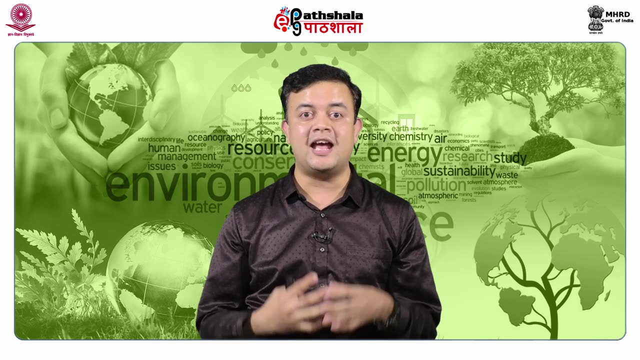 So unsustainable use of agriculture and fishing is driving a number of species to go extinct. So, in summary, the process of extinction, along with the speciation, determines the number of species that are going to go extinct. In public perception, most of the extinction that have happened in 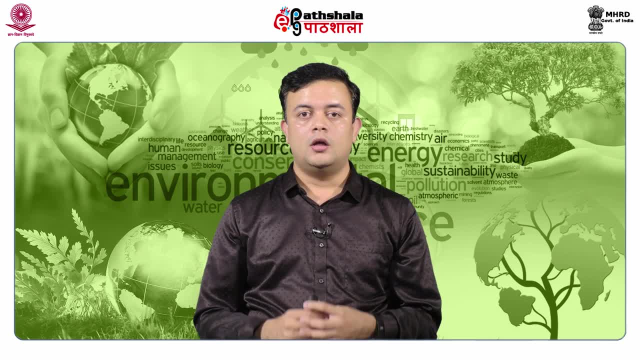 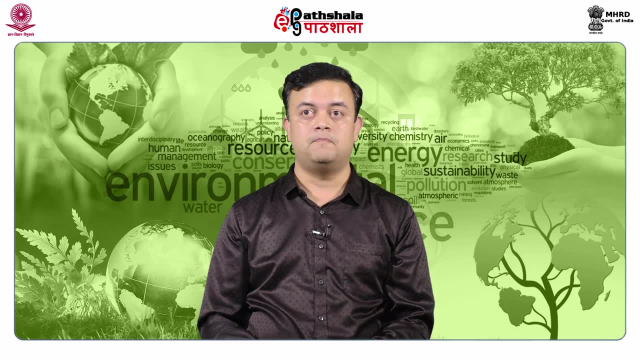 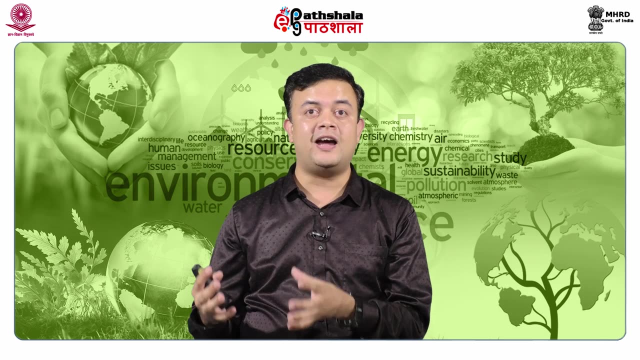 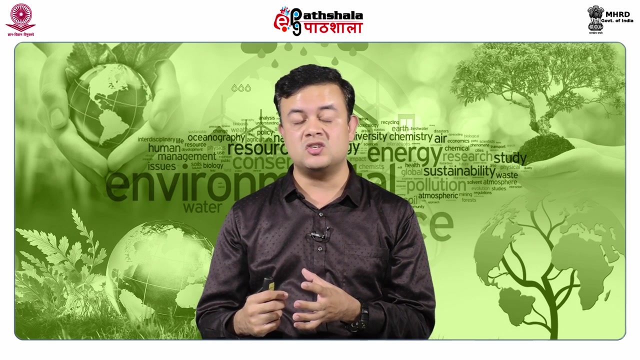 the history of life on this planet was due to the natural causes, not mediated by the human beings. Extinction is different from pseudo extinction and extirpation. Natural mass extinctions resulted in the extinction of a vast number of species and masses, So four 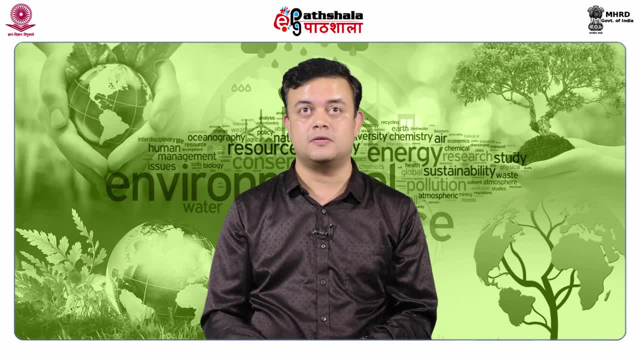 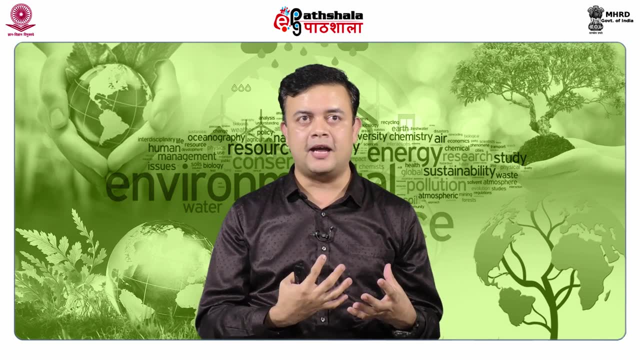 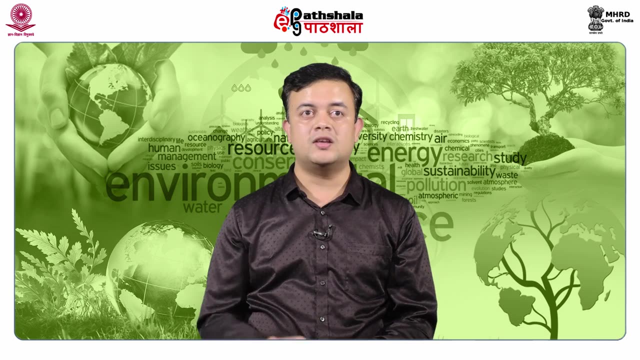 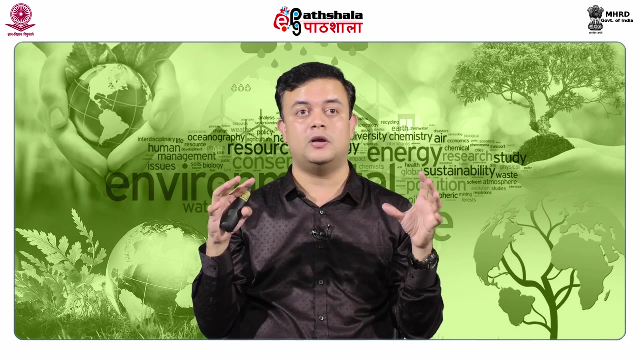 out of five extinctions was caused by increased rate of the extinction- species extinction, while one is caused by increased decrease rate of the speciation. Each of the five mass extinctions in the world is a consequence of the extinction of all species and all animals. 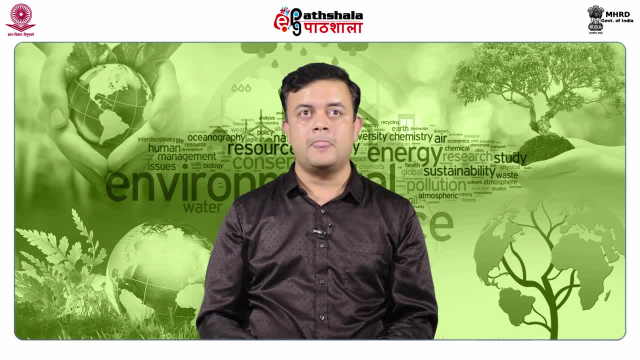 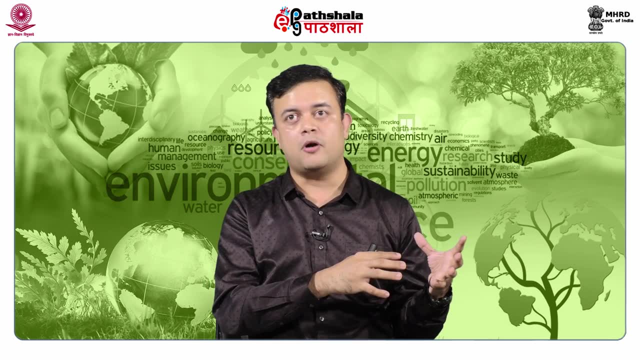 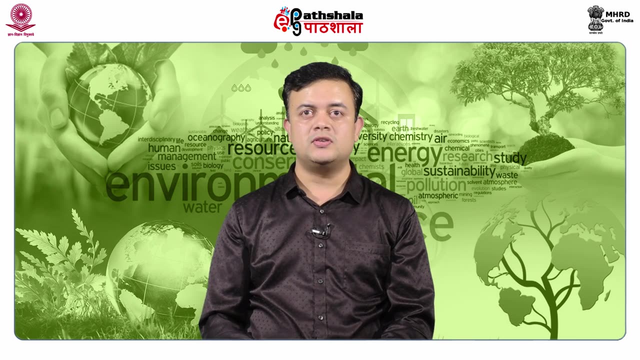 In fact, there is a consensus among the geologist and paleontologist that, since the beginning of the industrial revolution, the habitat loss, invasive species pollution, human population and over-harvesting for the resources summarized in the acronym HIPAA. 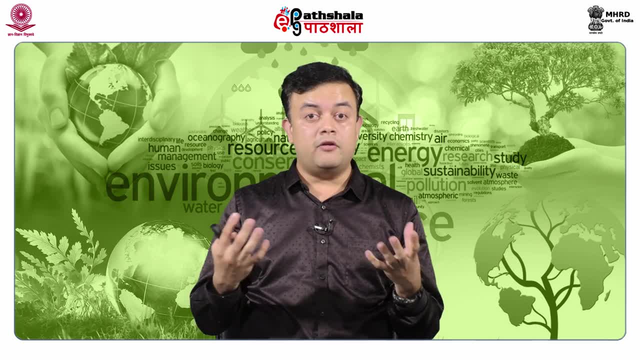 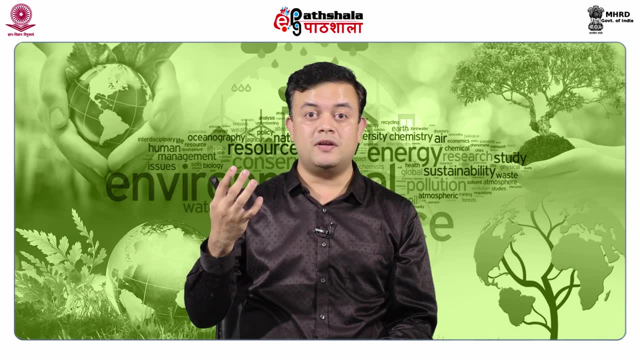 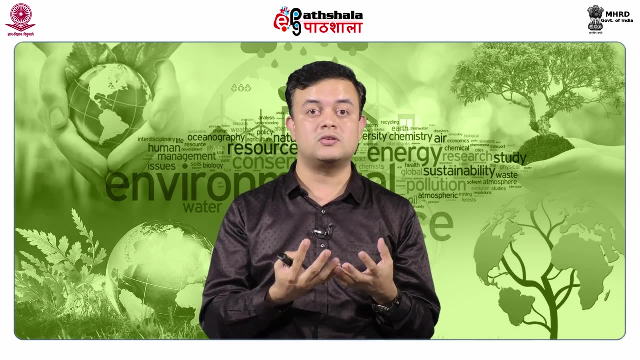 So, in summary, species extinction is a very, very important driving factor that determines the global diversity at any given point of time. Mass extinction events are extremely rare, but these are very, very important and most of these mass extinction events, the initial cause- we are not really certain. 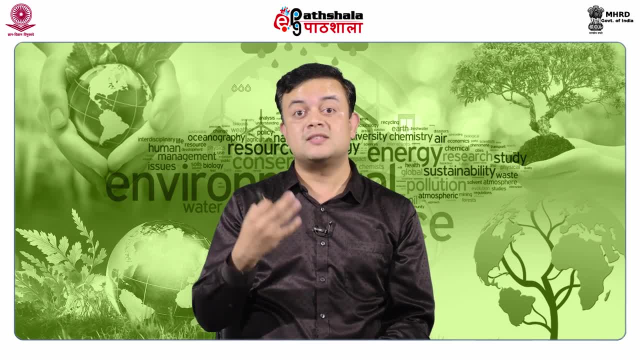 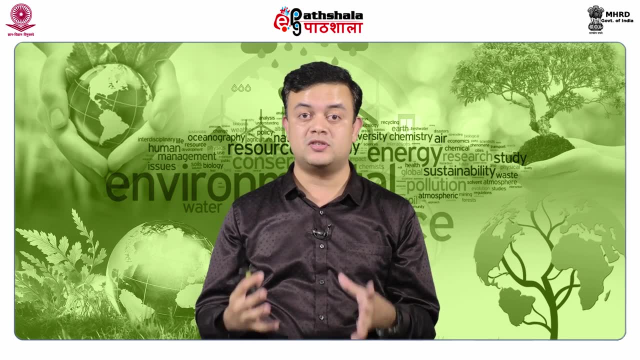 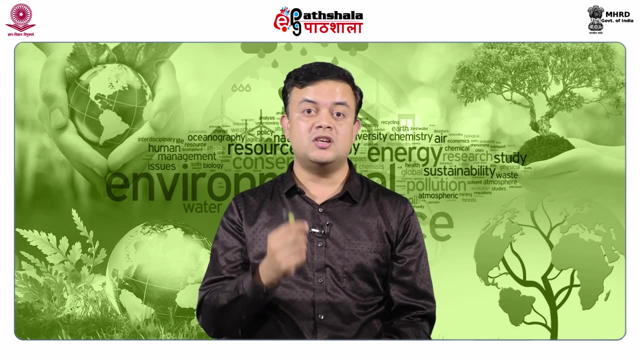 And the Earth is currently undergoing the sixth mass extinction event, called HIPAA. that is mainly driven by the human-mediated- so the current epoch is called Anthropocene- or because of the human-mediated anthropogenic activities, that is driving a number of species to go extinct.